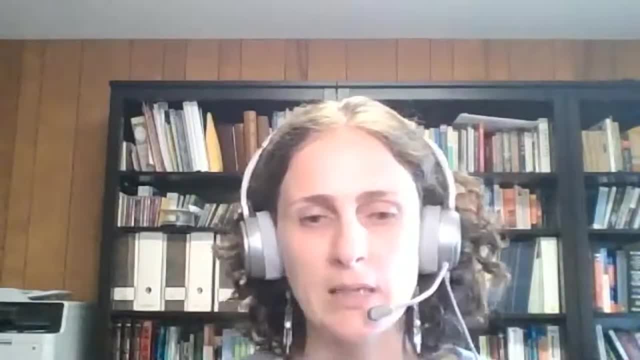 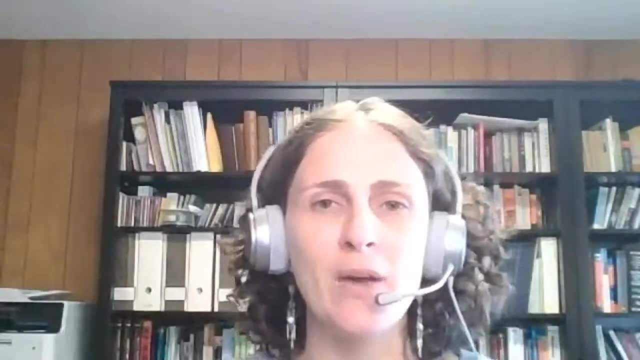 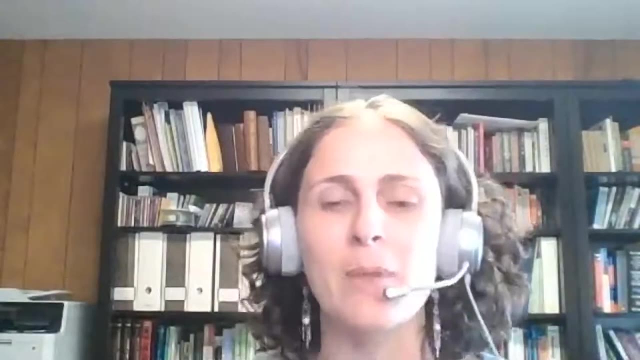 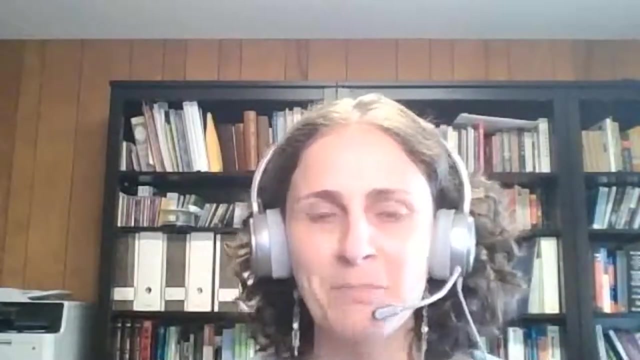 I have a bachelor's degree in computer science from MIT and a PhD in theoretical linguistics from Berkeley, And actually while I was at Berkeley I was in the US, I was teaching, so I like this kind of setting, although I haven't done it in a long time. so I'm a little bit nervous, and when I'm nervous I tend to speak fast. so if I'm too fast, feel free to stop me and ask me questions, okay. 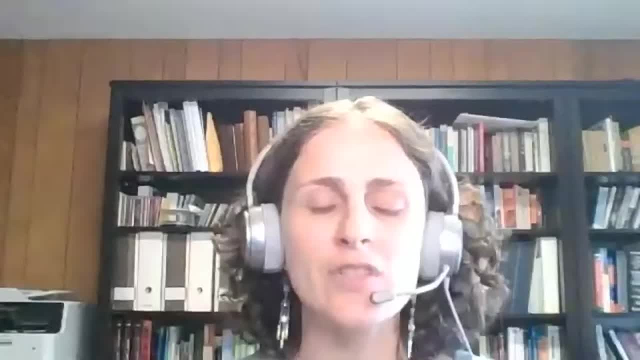 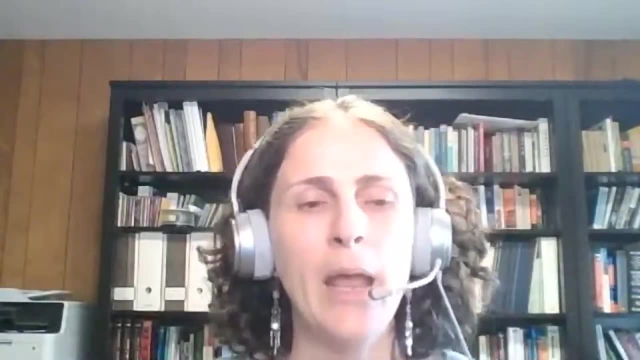 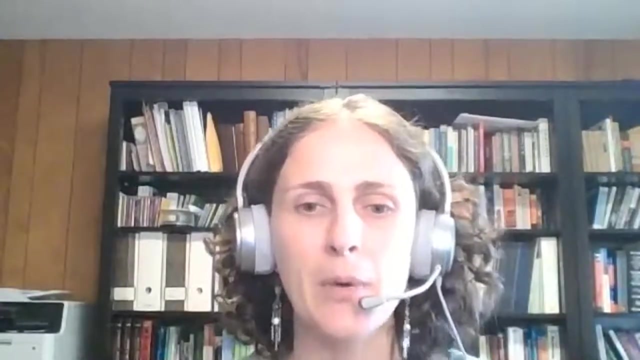 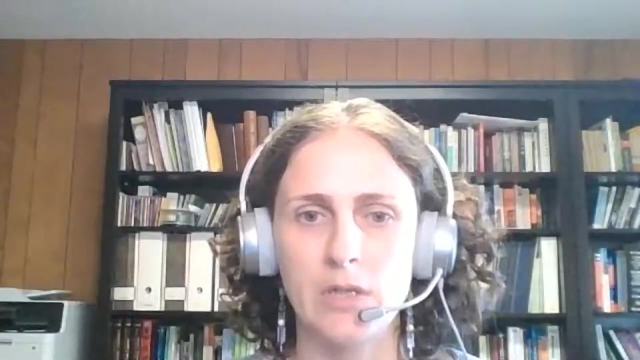 Okay, thanks a lot. Okay, So after I graduated from Berkeley, I worked for FactSet- It's a financial software company in the NLP group, and now I have my own consulting business In NLP, So I'm going to share my- let's see my- presentation. 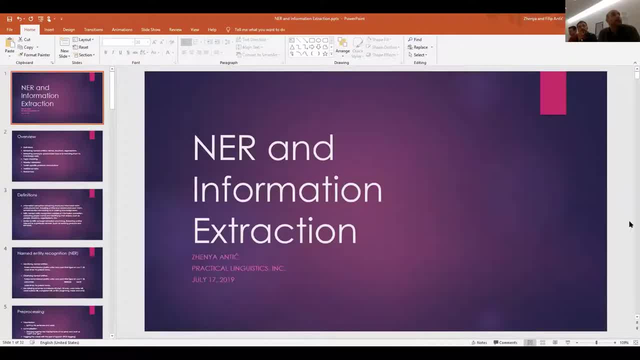 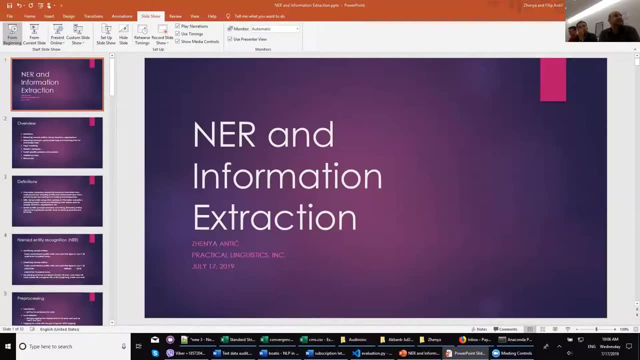 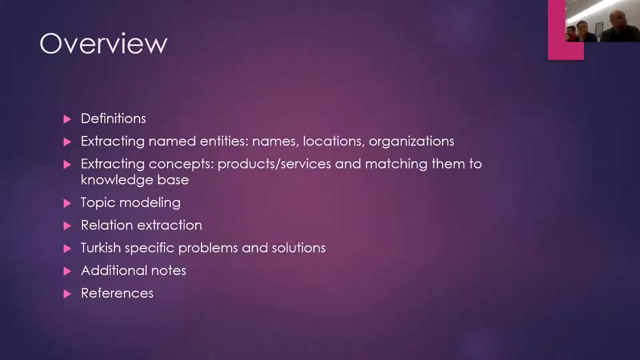 Can you guys see it? Yes, Yes, Okay, great. So now I'm going to start the presentation. Where is it Slideshow? Okay, so just an overview of what I'm going to talk about. I'm going to give some definitions. 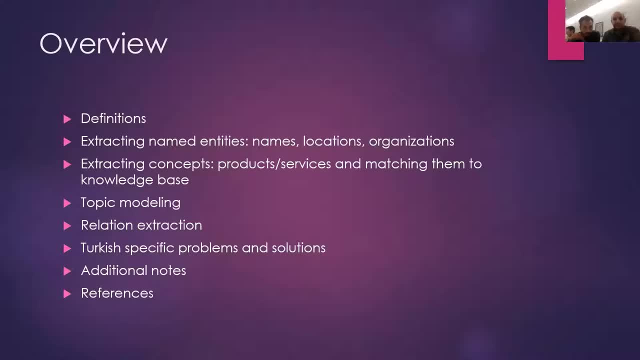 So I wasn't sure what you guys know, what you don't know. so if something is basic, I'm sorry If you guys know some things already, I'm sorry that I included it, but I wasn't sure what people knew and what people didn't know. 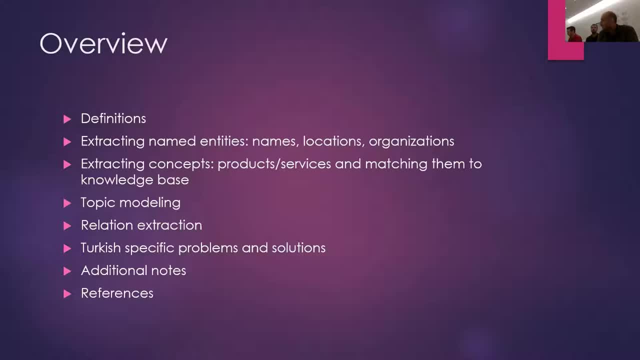 Then I'm going to talk about extracting, Extracting named entities, such as name, locations, organizations, Extracting concepts, such as products and services, and matching them to a knowledge base, Topic modeling, so putting together similar words and phrases. 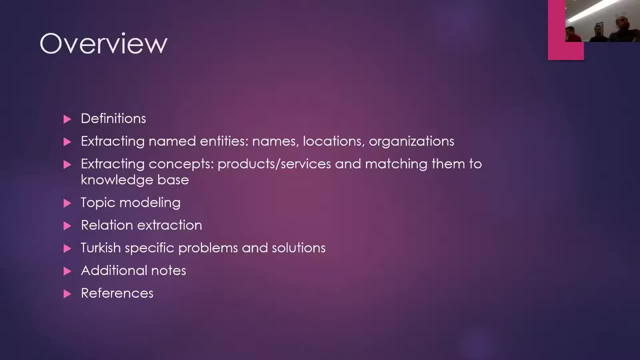 Relation extraction between entities. I did a little bit on Turkish-specific problems and solutions but I think actually with the modern tools Turkish is pretty well taken care of, so it's not a big deal. I have some additional notes. I went to a NYC NLP meetup yesterday and there's some interesting- a couple interesting notes that came from those talks. 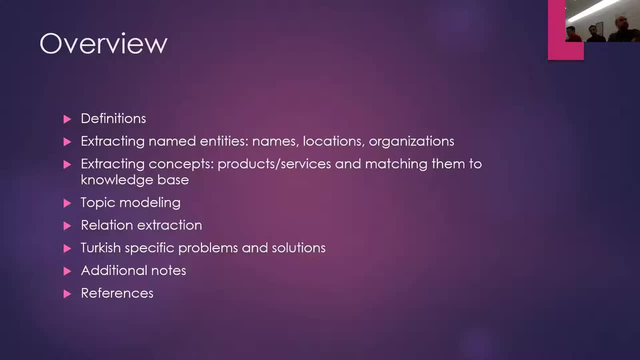 So I'm just going to talk about that as well And I included the references and you guys can go through. They're very detailed, very good references and you can use them when you work if you need to. So Just a few definitions. 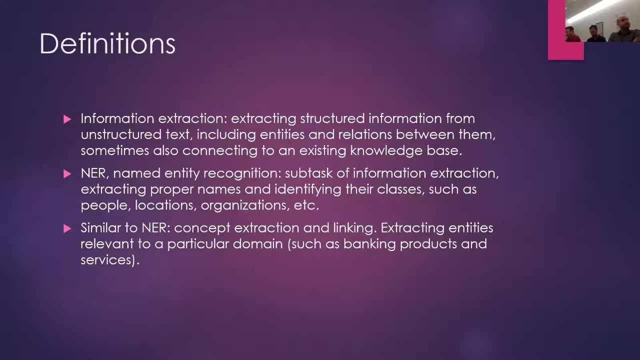 Information extraction is extracting structured information from unstructured text. So you're including entities and relationships between the entities, And sometimes you also want to connect to an existing knowledge base, And a knowledge base can be any kind of knowledge base. It could be Wikipedia, or it could be a custom knowledge base, etc. 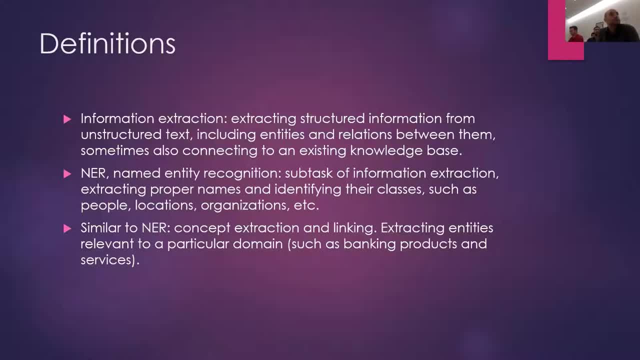 And NAR named entity right. Entity recognition is a sub-task of information extraction where you are trying to get the names, the locations, the organizations And you might connect them also to an existing knowledge base. Similar to NAR, NAR is concept extraction and linking. 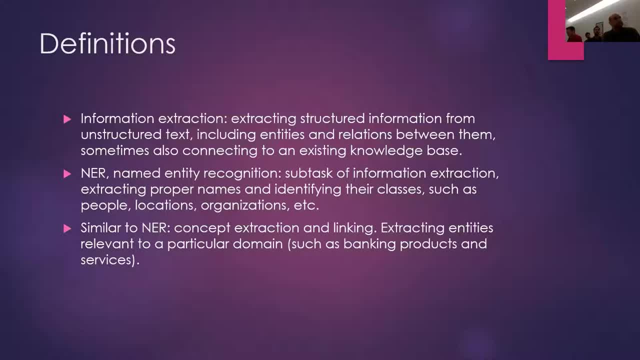 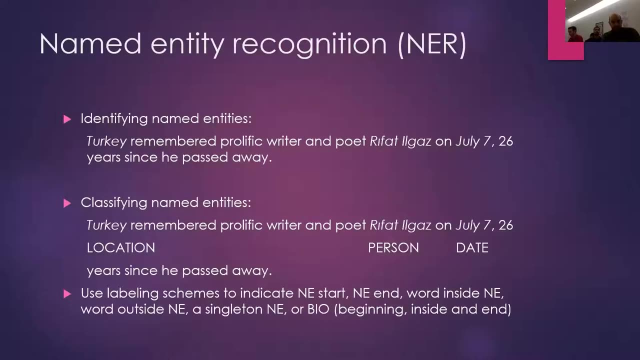 Basically, you're extracting entities, but they are not no longer named entities. they're no longer proper names, They're just concepts relevant to a particular domain, Such as, for you guys, banking products and services. So let's start with named entity recognition. 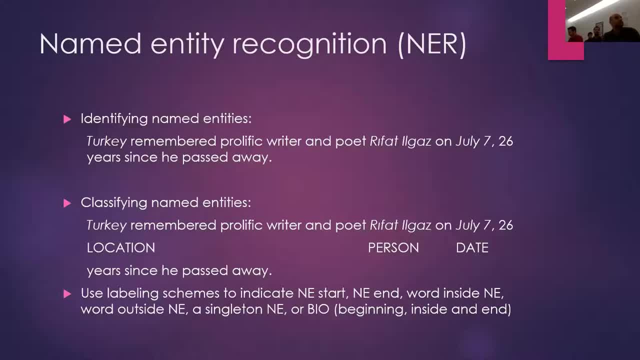 Again. you probably all know this, So you first identify named entities in a sentence Such as this sentence that I took from some website: Turkey remembered prolific writer and poet Rifat Ilgaz on July 7th, 26 years since he passed away. 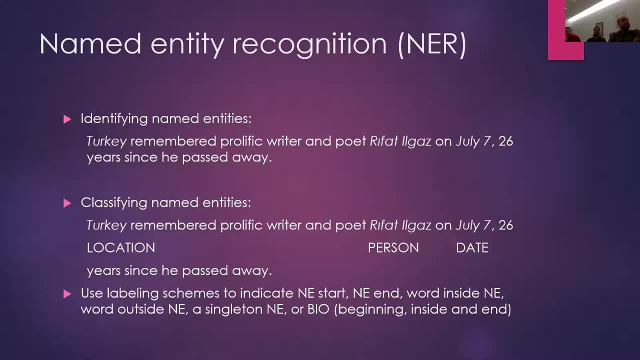 So first we want to identify where the names are, Where the named entities are, And then, once we have identified the named entities, we need to classify them. Here we classify them as location, person and date, And obviously the way we classify them differs from domain to domain. 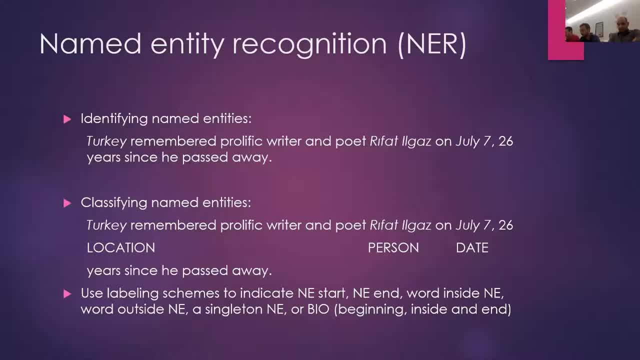 Some domains can use this generic classification, such as location, person, date, organization, etc. But others will probably need other names, Other classification schemes, More detailed or less detailed, Or others that include other classes, etc. And usually the labeling schemes indicate named entity start, named entity end and a word inside named entity. 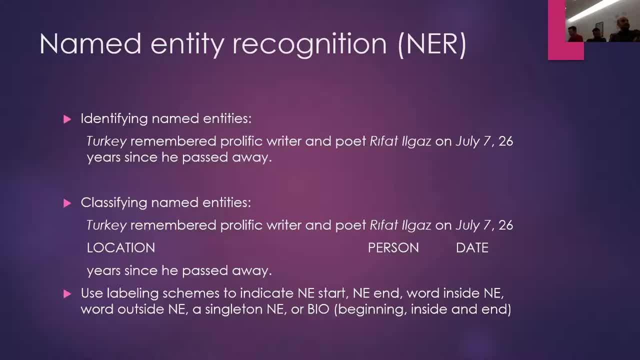 And words outside named entities. Or you could just say beginning inside and end, Sorry, beginning inside and outside, And then you don't really need to identify start and end, Because if you see an outside tag after an inside one, you know that the named entity stopped. 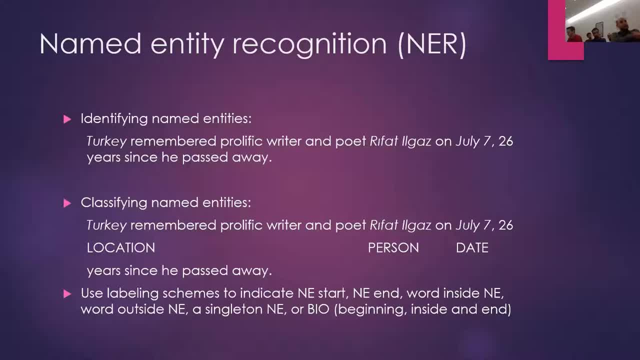 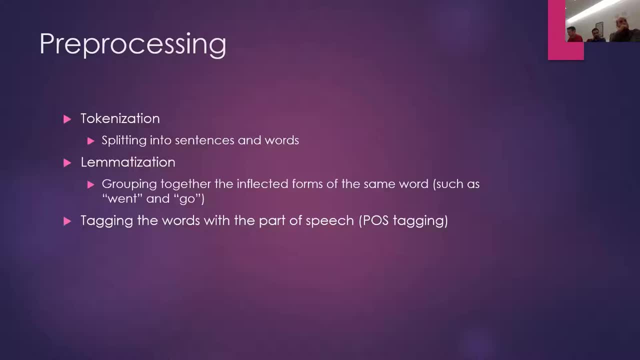 So basically, there are two different schemes. One is this one with three labels And the other one with five. And before you do NER, you need to do some pre-processing, Which is tokenization. obviously You need to split into sentences and words. 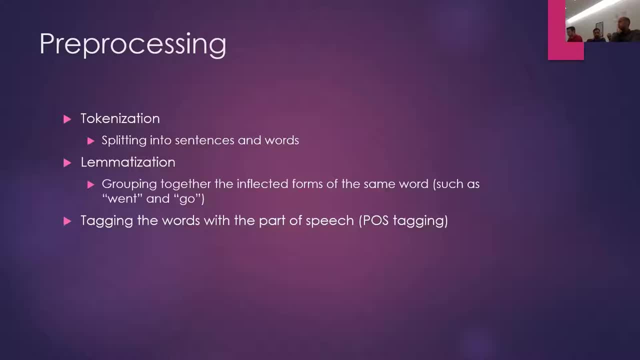 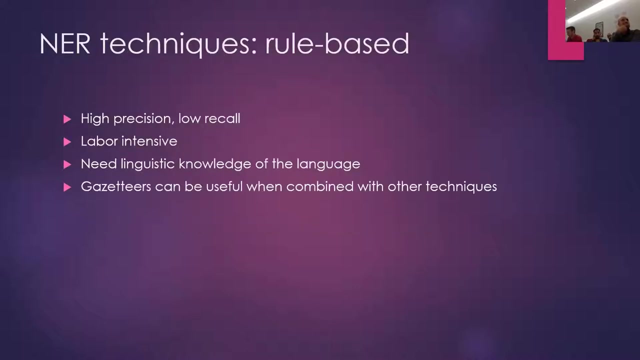 And then you do lemmatization, or grouping together the inflected forms of the same word, Such as went and go, And you tag the words with the parts of speech: QS tagging. So obviously for any kind of NLP task, for most NLP tasks, I should say: 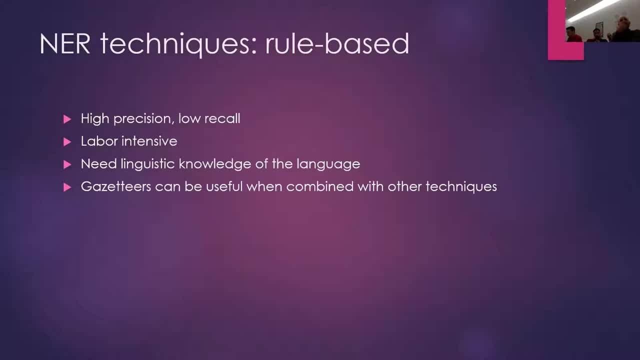 There's going to be three different ways to approach this. Right, You have rule-based approaches, You have machine learning approaches And you have deep learning approaches, where you don't need to engineer the features. So rule-based approaches apparently still exist for NER. 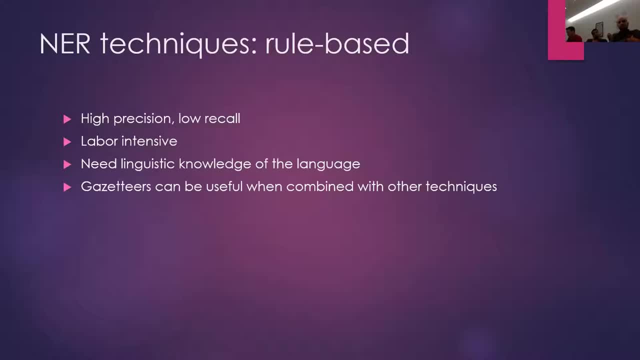 And they are high precision and low recall because they're very exact, But they're also very labor intensive, obviously, And the person engineering the rules needs to be very precise And the person engineering the rules needs to have detailed linguistic knowledge of the language. 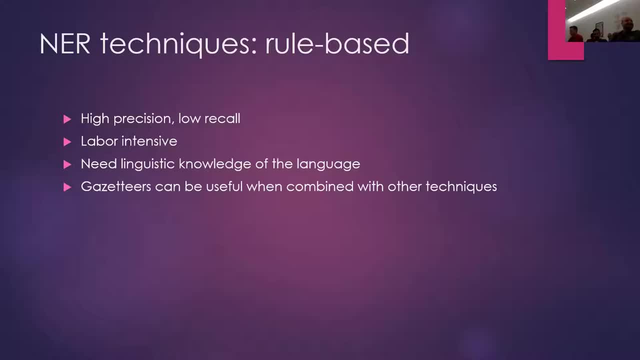 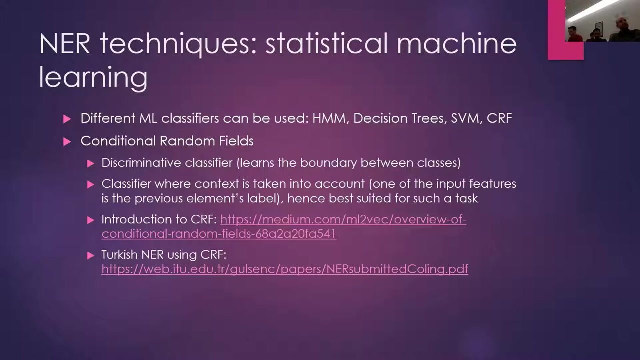 But one useful feature are gazetteers, or basically dictionaries. That can be combined with other techniques such as statistical machine learning or deep learning. So statistical machine learning techniques are now basically the most common way of how NER is done, And different ML classifiers can be used, such as decision trees or SVMs. 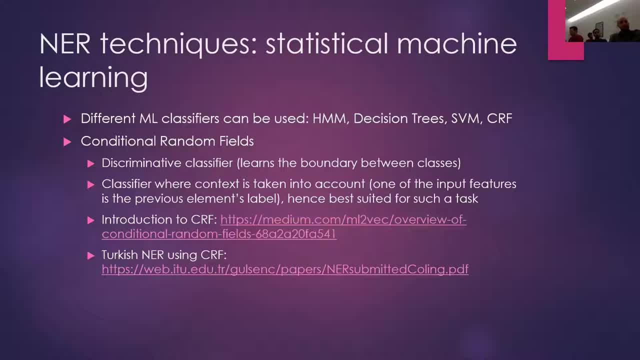 And the standard one which I saw throughout the literature was conditional random fields, Which is a discriminative classifier, since it learns the boundary between the classes And the reason why conditional random classifiers are used for NER and similar tasks, such as where there's a sequence of 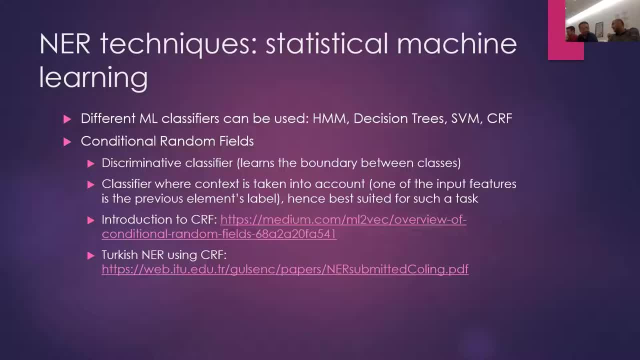 Of words or something else. where you need to label a sequence is because you take into account context, So it's best suited for such a task, for a sequence labeling task. So you have some links here. And there is actually Turkish named entity recognition using CRF. 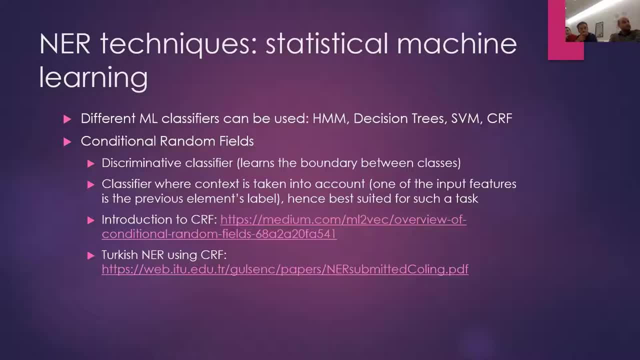 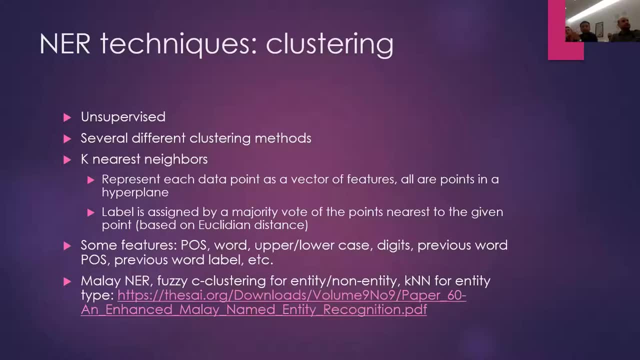 So you guys can take a look at that. Now you can also use clustering for named entities, So you can use entity recognition, which is unsupervised, And you just cluster similar entities together. And there are several different clustering methods. One of them is k-nearest neighbors, where you represent each data point as a vector of features. 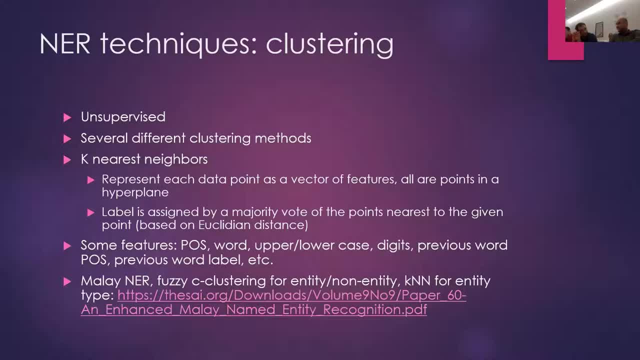 And all are points in a hyperplane, And then you compute this Euclidean distance between points And then the way a label is assigned to a point is that points closest to that one point give a majority vote on what the class is, And some features that are put in as input are part of speech. 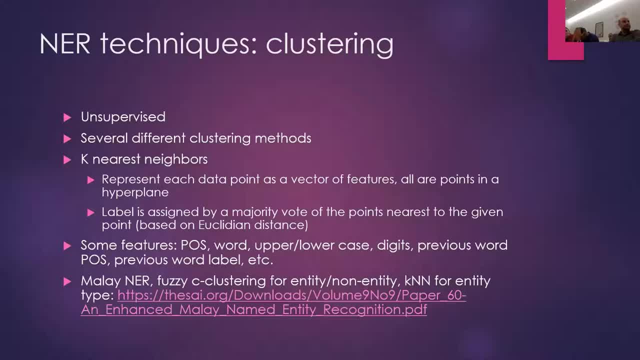 the actual word, upper or lower case digits, previous word, part of speech, previous word, label, etc. So there is a paper on. There is a paper on Malay named entity recognition, which uses two different clustering methods for first identifying whether it's an entity or a non-entity. 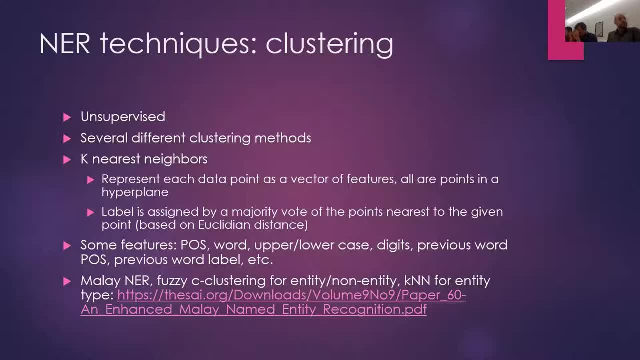 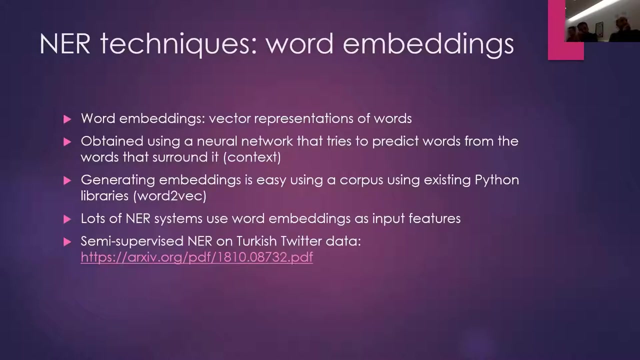 and then labeling the entity type. So it uses fuzzy C-clustering, some other kind of clustering method for identifying whether it's an entity, and then k-nearest neighbors to label the actual type. So the trend of course has been lately is to use word embeddings throughout NLP tasks. 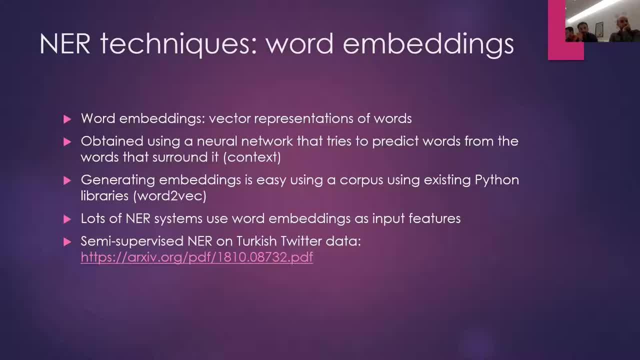 and named entity recognition is not an exception. So, basically, we represent words as vectors in word embeddings, And they are obtained using a neural network that tries to predict words from the words that surround it, And you can easily, I mean I'm sure you know this- 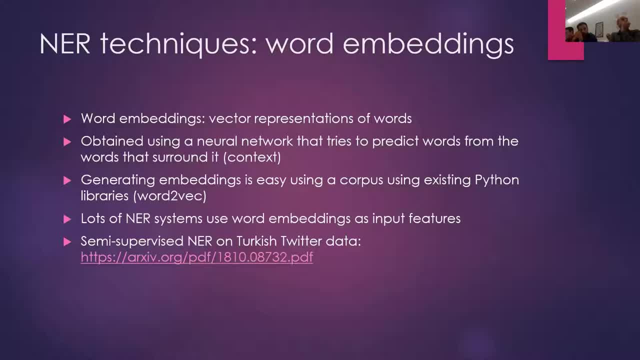 But generate embeddings easily using an existing corpus. with Python libraries And lots of named entity recognition systems use word embeddings as input features. Here you have a semi-supervised named entity recognition paper on Turkish Twitter data. It's a little different for Twitter data because it's very short text. 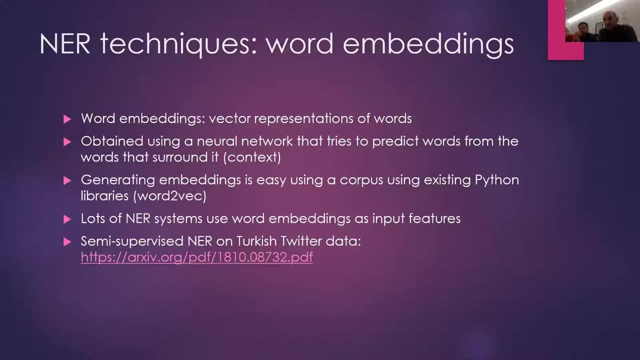 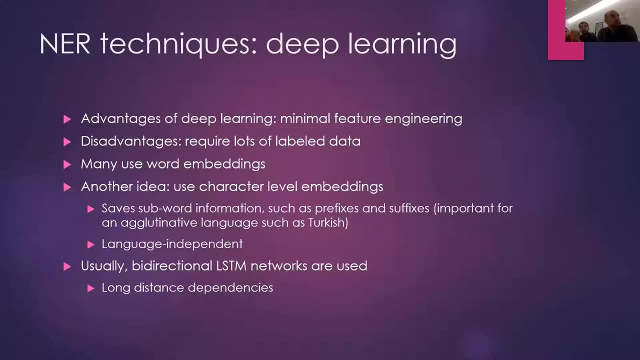 They don't have much context but it's relevant nonetheless. And of course there are deep learning approaches to named entity recognition And advantages of deep learning is that we don't need to engineer the features as we do for statistical machine learning, But a disadvantage is that it requires lots of labeled data. 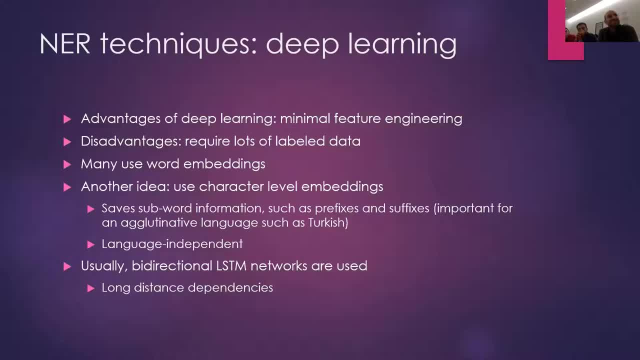 Many deep learning methods use word embeddings as input, or at least part of input, And another idea is not to just use word embeddings but also character level embeddings, So it saves sub-word information such as roots and prefixes and suffixes, which is important for an agglutinative language such as Turkish. 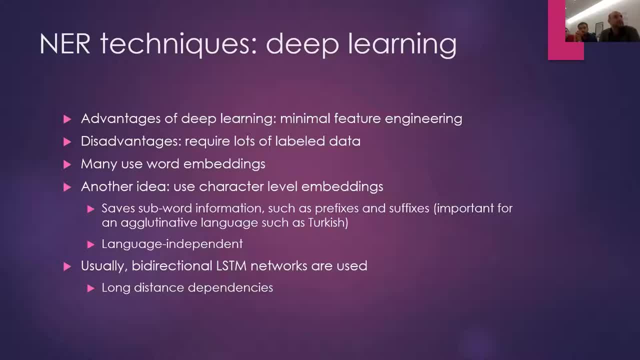 And also such approaches can actually be language independent, since you just go character by character, And usually bi-directional. long, short-term memory networks are used because they take into account long-distance context dependencies And the state of the art. basically, as far as I understood. 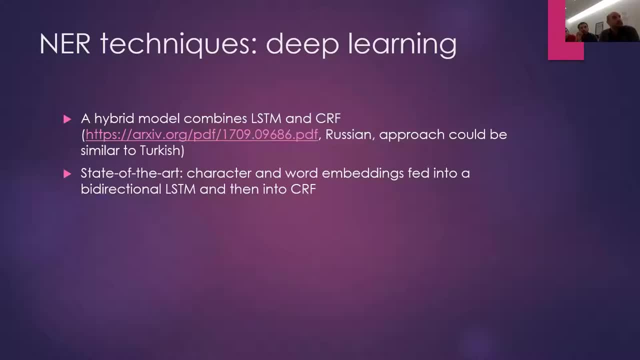 is you use character and word embeddings and you feed them into a bi-directional long short-term memory network and then into a conditional random field. So there's a paper on using such a model for Russian and the approach is similar, because I think Russian and Turkish are similar. 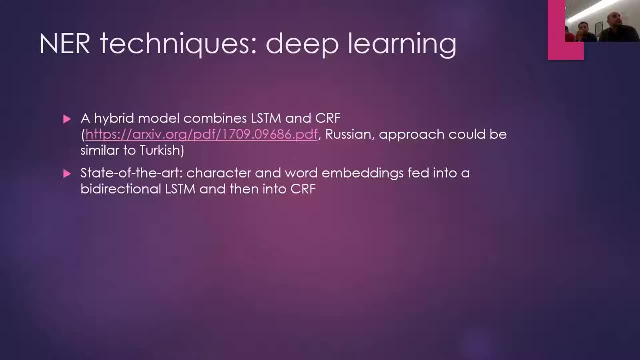 because they're morphologically rich. So I think that's it on NER. Do you guys have any questions on that? Do we have a question here? No, I don't see any hands, so we can proceed. Okay, sounds good. 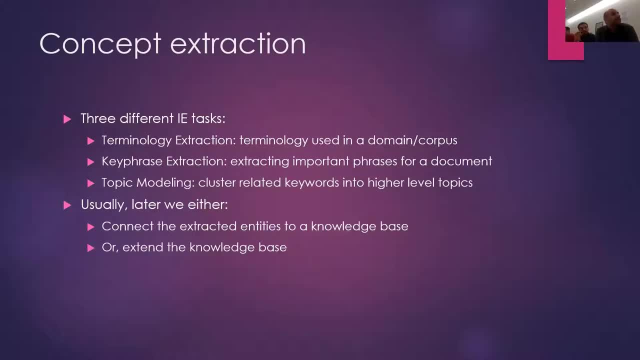 Concept extraction. It's similar- somewhat similar- to named entity recognition, in the sense that you're extracting entities, but it's also a little different. And the three main tasks under concept extraction are: terminology extraction, where you have a corpus already and you want to find out. 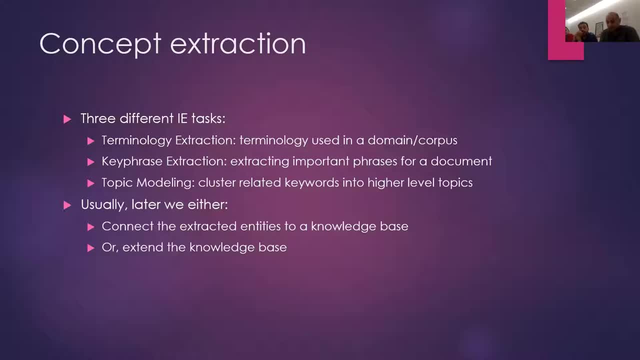 what kind of terminology is used in this corpus or in a domain. Then you have key phrase extraction, which is: you're focusing on a document, what kind of terminology is extracted from a document? And then you also want to use topic modeling to cluster related keywords into higher level topics. 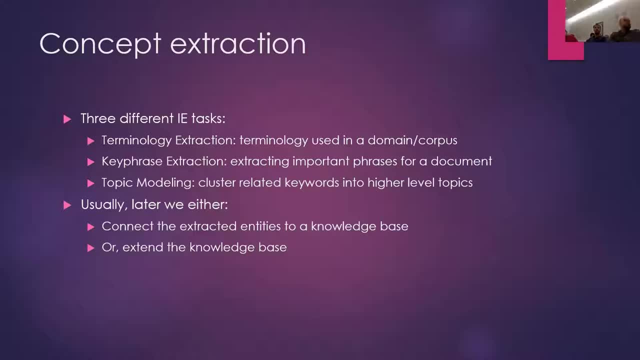 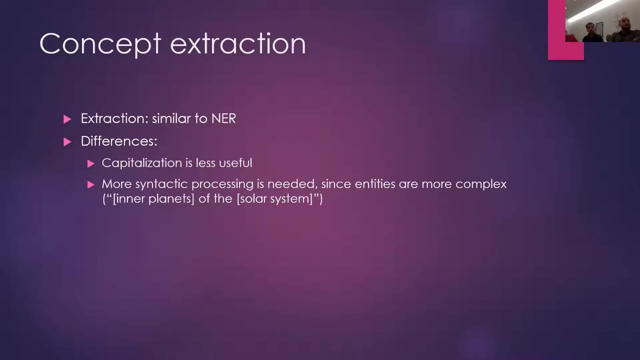 And then, once we extract concepts, we want to either connect the extracted entities to a knowledge base or sometimes we want to extend the knowledge base because we found some new concepts that are not in the knowledge base. So again, it's similar to named entity recognition. 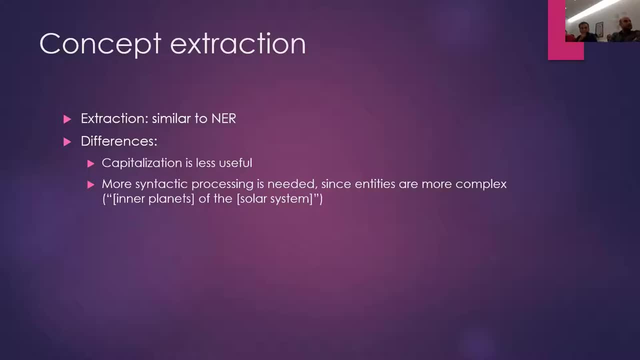 but differences are is that capitalization obviously is less useful And it's more complex because you don't have. sometimes you have bigger entities that have more words, such as here, inner planets of the solar system, And actually the whole thing is also an entity. 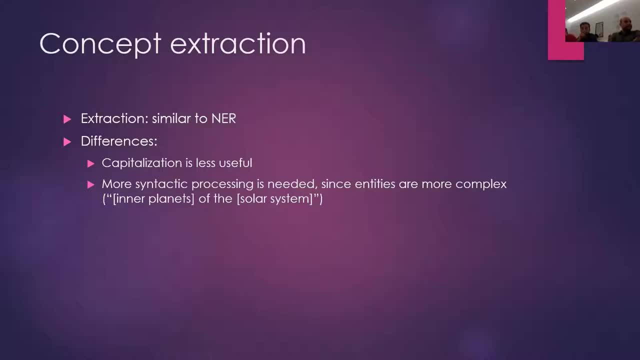 Inner planets of the solar system. So how do? first, we need to find candidate entities, And the way to do the approaches that are used is: one is extracting n-grams to a predefined length, And another is you need to do some kind of shallow syntactic parsing. 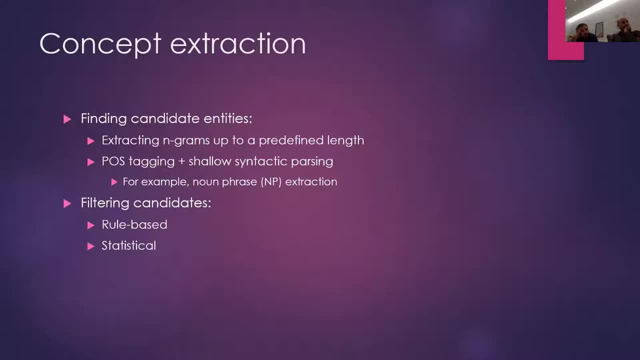 and extract noun phrases, And you of course need to first do part of speech tagging to find out what are the parts of speech, And then, once you find candidate entities, you filter them, either using rule-based systems or statistical systems. So for statistical systems, once you want to filter, 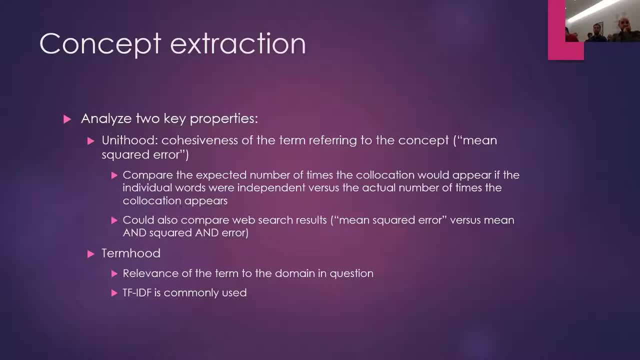 you analyze two key properties. The first property is unit hood. So it's: how well do these words stick together basically? So compare the expected number of times this collocation, such as mean squared error, would appear if the individual words were independent. 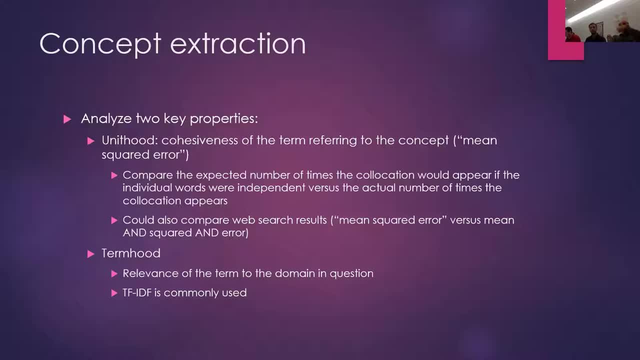 versus the actual number of times the collocation appears. So if the words were independent, it would appear less because mean squared error. what are the chances that those words appear together? But since this is a unit and it appears more actually, Or you could also compare web search results. 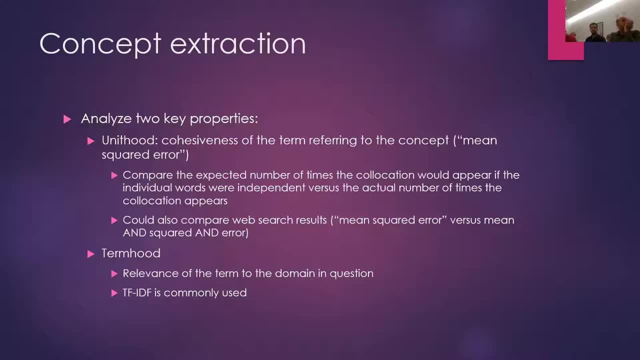 for mean squared error in quotes. so just for that term versus for mean and squared and error, Although I'm not sure how it actually works with Google nowadays. I'm not sure if that actually works, But it was reported in one of the papers. 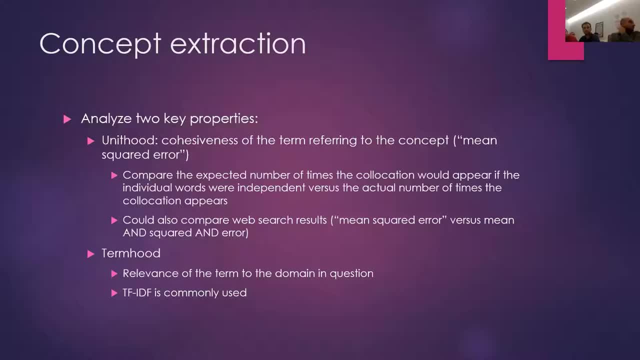 And the other key property is term hood, which is relevance of the term to the domain in question, And here TFIDF term frequency- inverted document frequency- is commonly used. So basically, if the term is frequently used in the document but infrequently used across other documents, 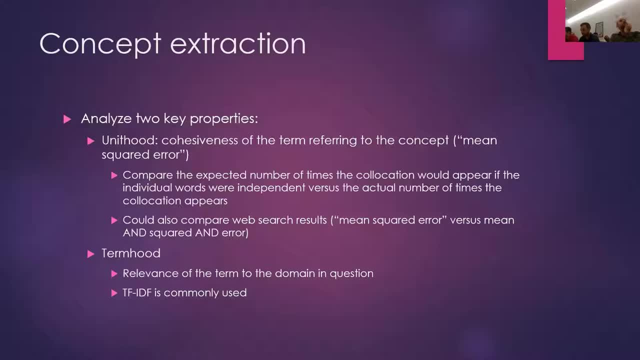 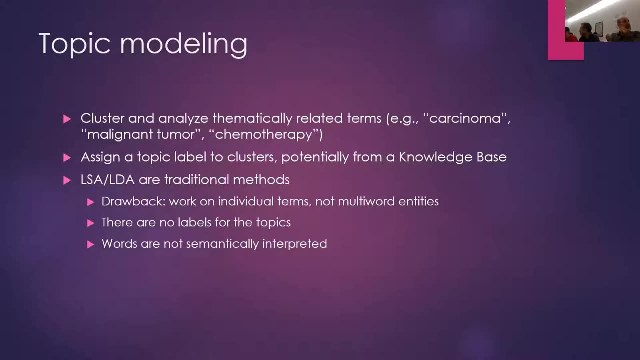 that means it's relevant to this particular domain. Okay, so once we actually extract terms or topics from the document or domain, we want to sometimes group thematically related terms together, such as things related to cancer, for example, here, And we want to assign topic label to the clusters. 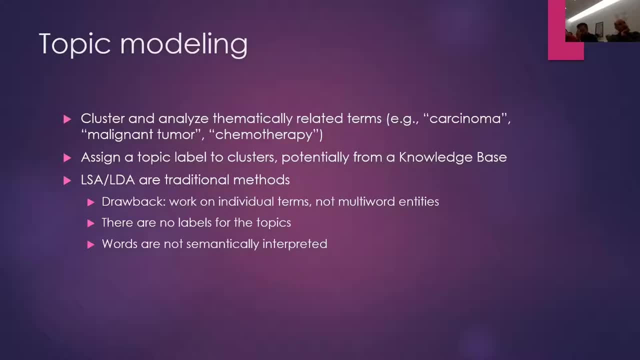 potentially coming from our knowledge base or an external knowledge base such as Wikipedia. So, for topic modeling, LSA and LDA are the traditional models, but they have some drawbacks, which is they work on individual terms and not multi-word entities And there are no labels for the topics. 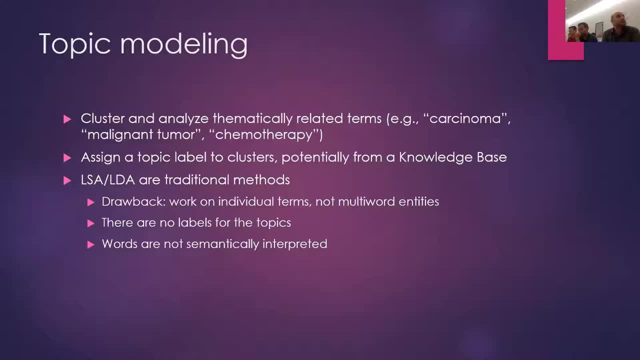 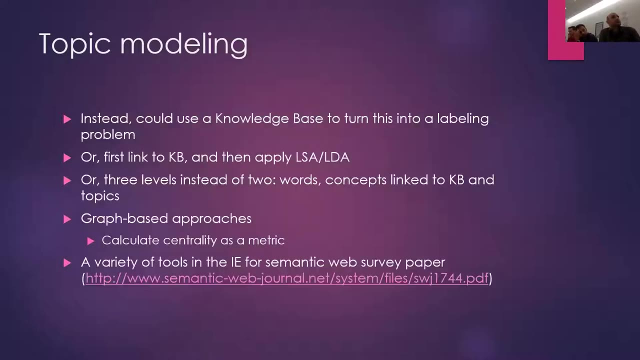 Basically, what comes back to you is our clusters, but you have to assign the name to them And the words are not semantically interpreted, meaning they're just used as a label and not any kind of meaning. There's no meaning in them. 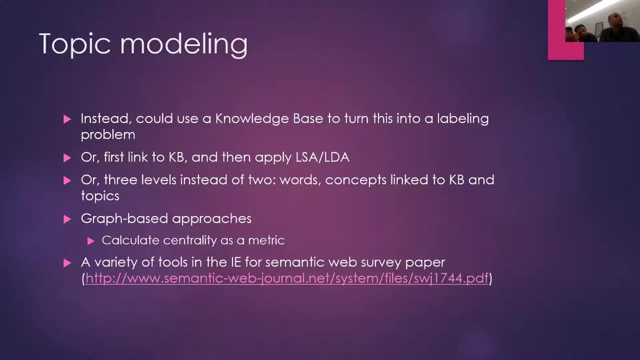 So there are, there are some other approaches to this and we could use our knowledge base to basically turn this into a labeling problem. Say we say, okay, so these are the topics that come from the knowledge base. How can we label these entities using our knowledge base? 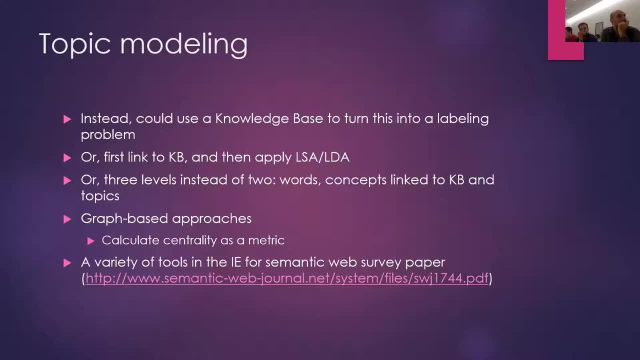 Or you could apply LSA and LDA after first linking to the knowledge base. You could also use three levels of instead of two, where you have the words, you have the concepts linked to the knowledge base and then you have the topic. 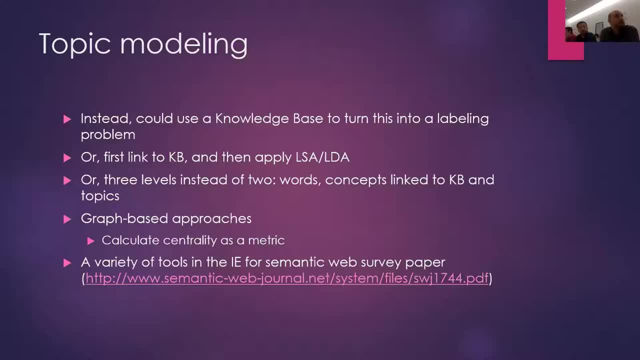 Excuse me, And then I actually saw a trend to use graph-based approaches as a like, an emerging one. They're being used more and more, it seems to me. And you calculate centrality as a metric, And I'm not an expert in graphs. 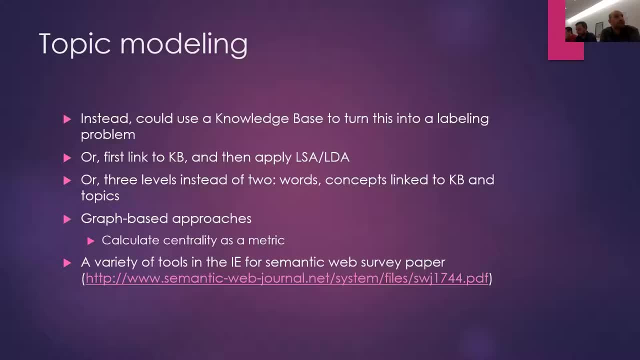 so, but it looked looked very interesting. So there are a variety of tools in this paper, which is also in the references. It's like a big paper that describes in detail, like all these things like named entity recognition and concepts and relation extraction. 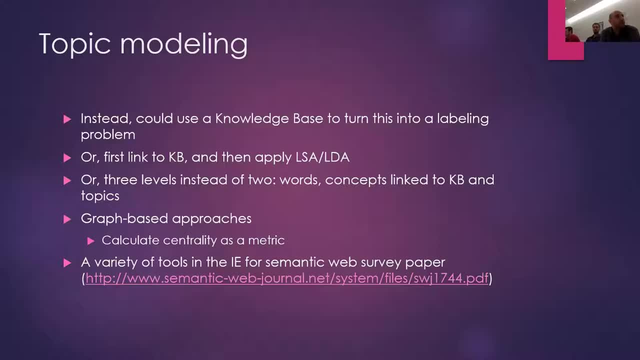 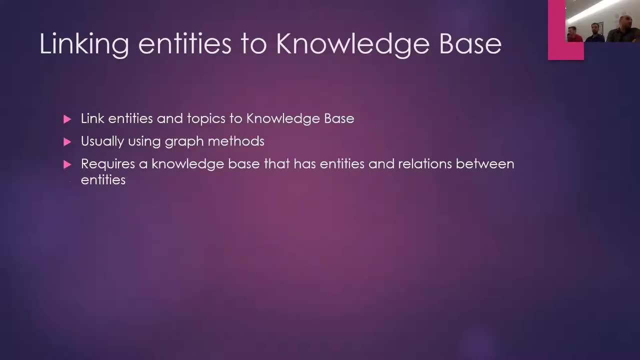 And then it compares all the tools on on how they perform. So maybe you'll find it useful. So how do we link entities To the knowledge base? Usually it's done using graph methods and require it obviously requires a knowledge base that has entities and relations between. 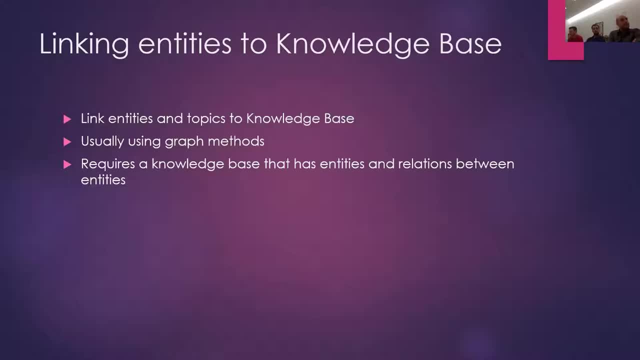 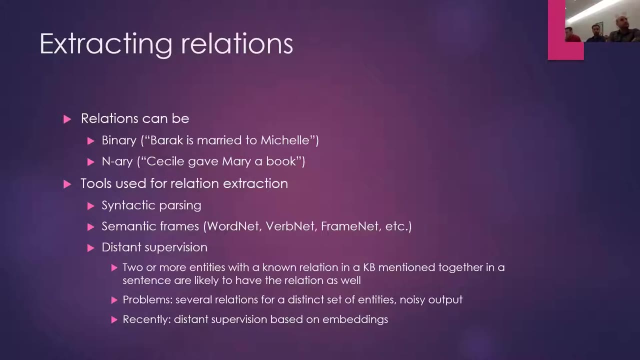 entities. And again you could use Wikipedia, which has a whole bunch of entities and relations, or you could use, like a specific domain, specific knowledge base. Okay, So how do we actually extract relations between entities? The relations can be binary. 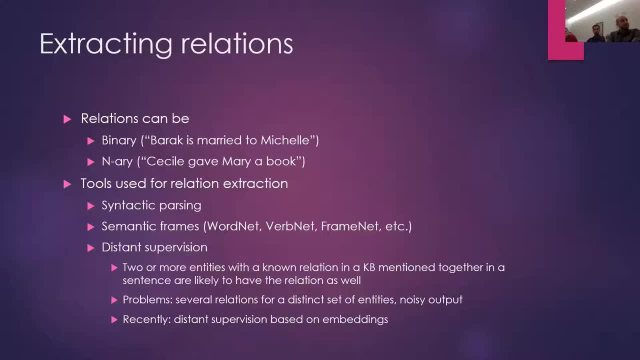 such as Barack is married to Michelle, whereas there's only Barack and Michelle, and it could be an Aerie or more than two, whereas Cecile gave Mary a book where we have three entities: Cecile, Mary and a book. 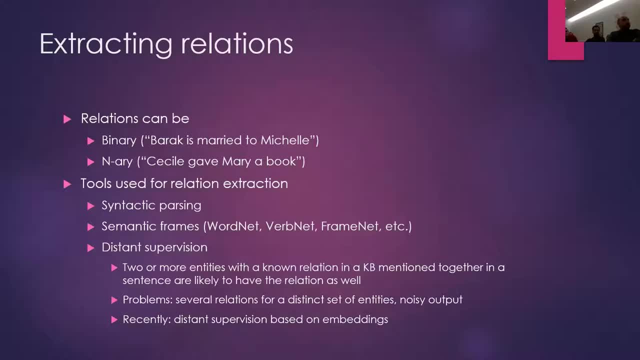 And tools that are used for relations extraction. obviously, again, we have the rule-based approaches, which are syntactic, parsing and semantic frames. So using those in conjunction or by themselves, And as always, that's, you know, this kind of moving away and it's kind of becoming a thing of the past. 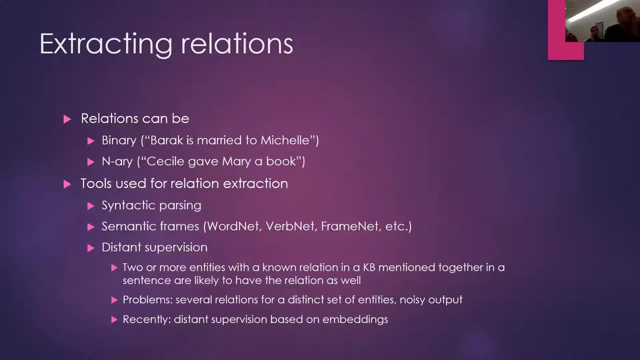 So the other approach is distance supervision, which is based on an idea that if we found two or more entities in a sentence that also have a known relationship in a knowledge base, then likely they have that relation relation in that sentence, which is: 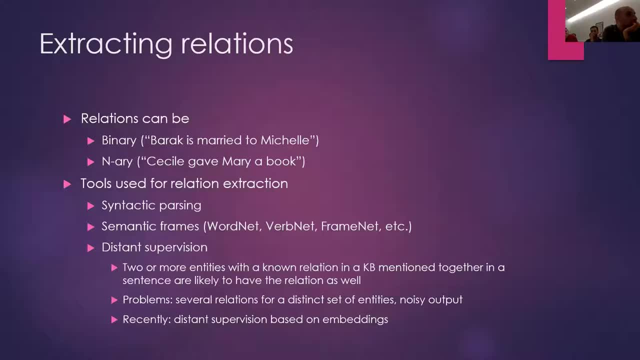 I mean it's a good idea, but it also results in a lot of noisy output And sometimes you have several relations for a distinct set of entities and you don't know which one to pick. And recently again, we see embeddings appear again and again. 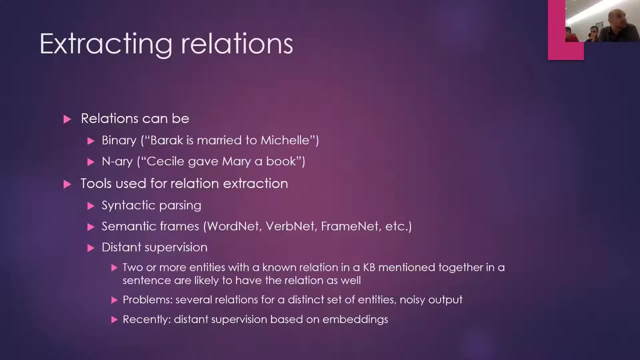 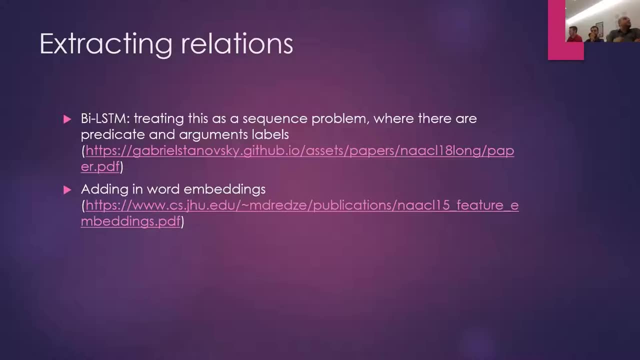 and distance supervision has been used with in conjunction with word embeddings, And since this is also could be treated as a sequence problem, where you take a sentence and you say, okay, so we have, Barack is married to Michelle. So then we say Barack is an argument. 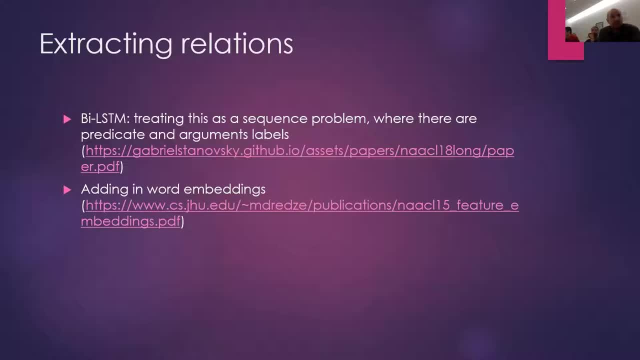 is married is a predicate, and Michelle is also an argument. So we have the sequence labeling. We take the sentence Barack is married to Michelle and we want to output a sequence of labels. So then again, bi-directional long. 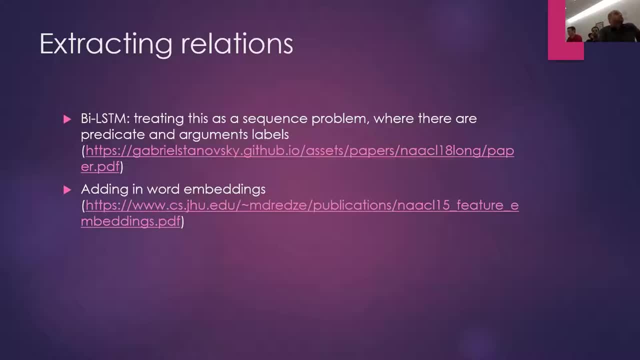 short-term memory model is a natural thing to use, because this is a sequence labeling problem. that also, and also a good thing about bi-directional, long-term, long-term memory models- is that they take into account long distance dependencies, not just immediate dependencies. And then there is a paper on adding in word embeddings. 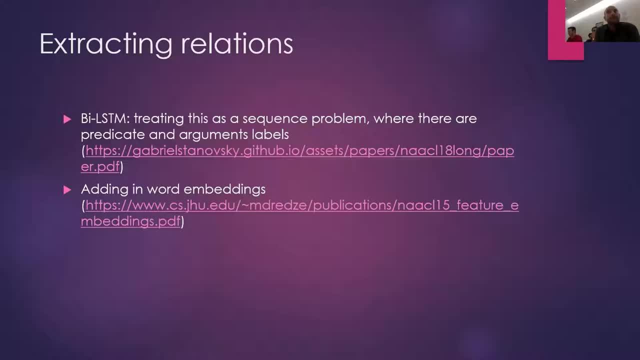 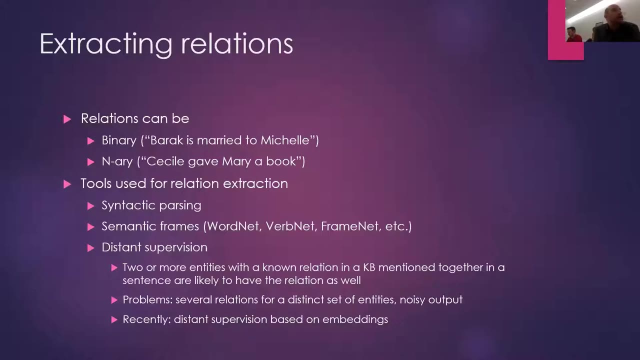 and I think it's used in conjunction with also LSTM There. Zahina, may I stop you here because I have some questions. Yes, Can you go back on the slide back This one? Yes, I need more examples how to do. 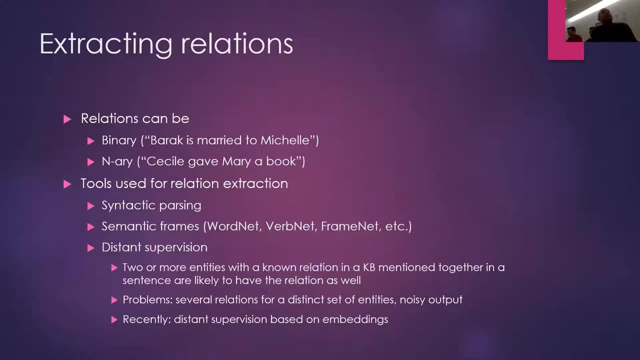 For example, first of all, we assume that there is a knowledge base, So for that I should train a graph, right Knowledge base graph, Assuming that I have it Right. So what you propose is like: okay, I have a knowledge graph between some entities. 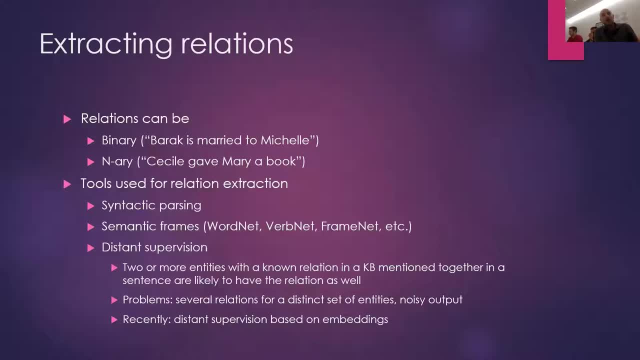 I have the relations Right. So how I'm going to use these to extract entities? or am I using the knowledge graph and assuming that I have NER model as well? So I know the entities in the sentence. So are you proposing that I can use this NER to create new relations in the knowledge graph, to improve my knowledge graph? 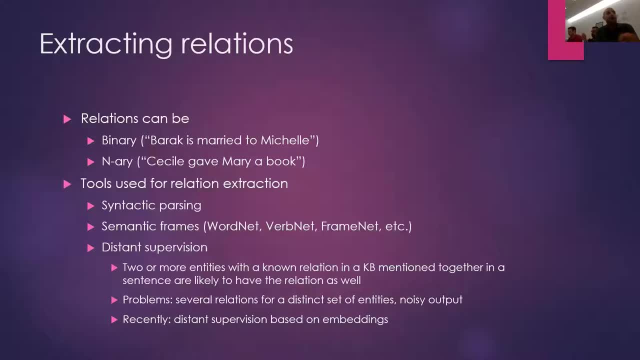 or you are doing other. I'm doing other way around. So I have a knowledge graph. given a knowledge graph which I should do it by myself. Like I cannot do it, Do I have a method? you know? So I think mostly the papers that I read, 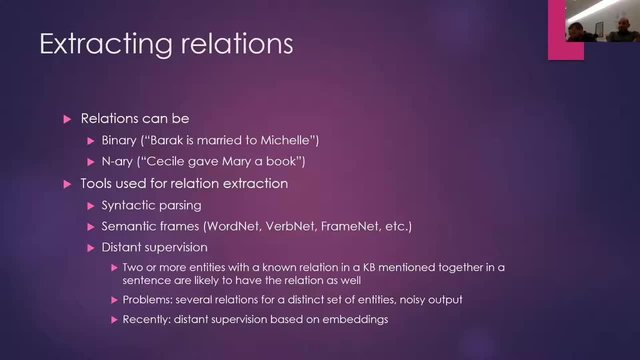 they mostly talk about matching the relations to an existing knowledge graph, But there you can also do probably relation discovery right, Like if you don't have a relation you can probably propose new relations If they're not in your knowledge base. So 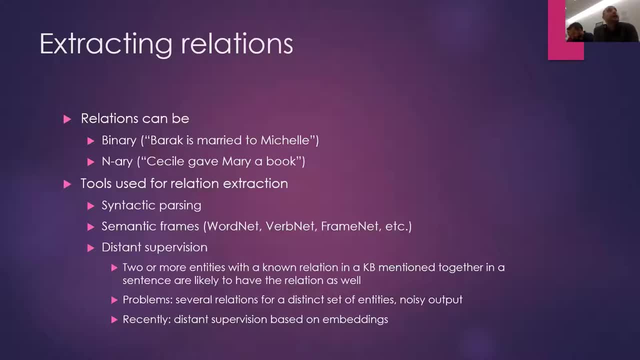 You're right. So the question like: when they say, okay, we have the knowledge graph, Normally they they pin it to the Wikidata knowledge graph. Wikidata, Yes, Wikidata. Have you seen the knowledge graph? You can. 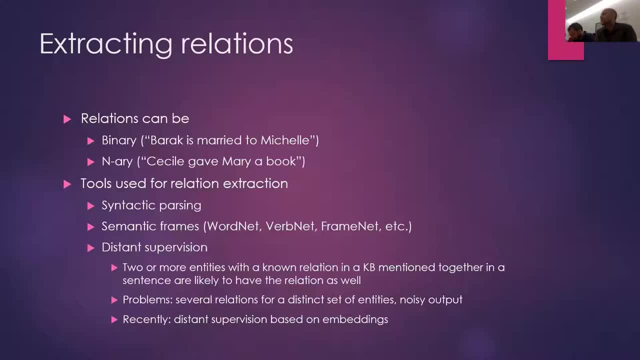 you can search some, you can put some queries like they have, Right Yeah, Do you have a like they have a, a specific, a specific language, so you can make queries, right Yeah. So, but the question is: 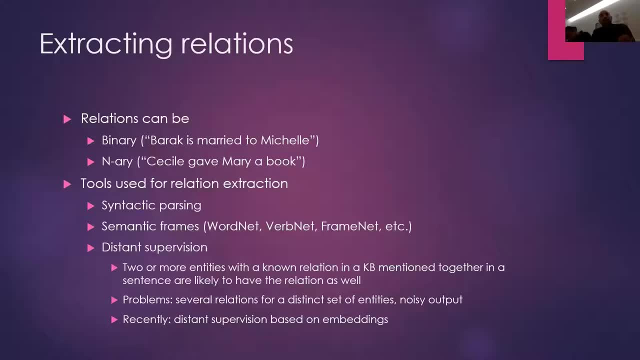 if I want to do it like Wikidata for banking, because we are. we are in the banking. we don't. we are not interested in all the information in the work, but we are interested in the banking domain. specific knowledge graphs. 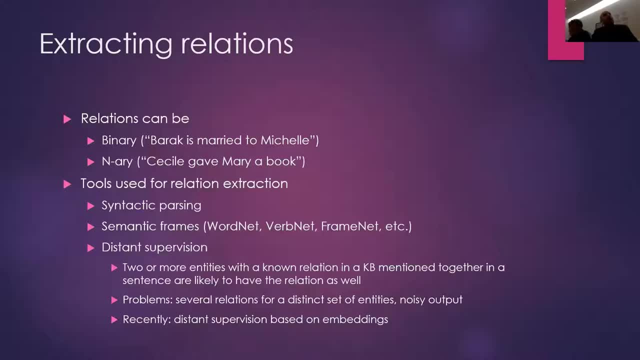 Right. So one way is okay. I, I have a bunch of thousand, thousands of the entities, Right. I start to create the some random, random relations between them. Then I or I have some corpus. I read the corpus and create some relations. 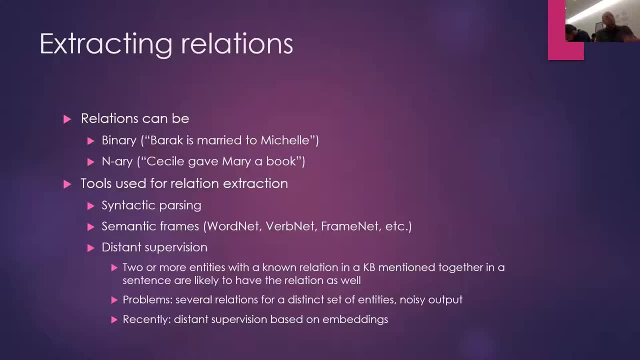 which is because- which is a very difficult task, I know Wikidata. they had a platform. They asked people to write about each entities, So then I, then, through the platform, they could recognize the, they could create the knowledge graph in the. 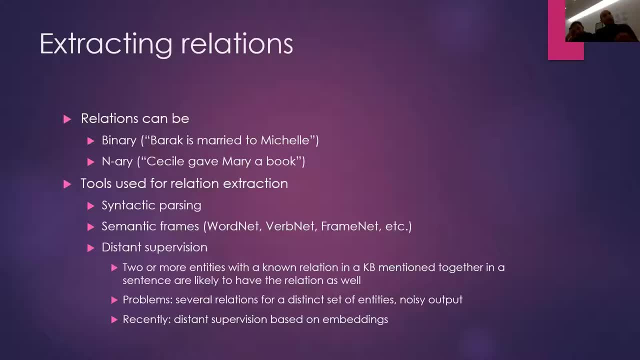 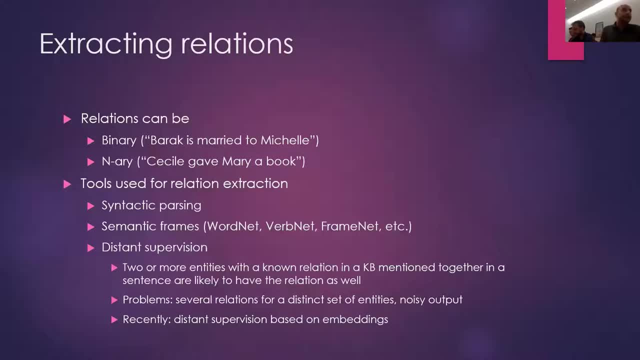 And they were writing people, that people were writing about any paragraph about Barack Obama. Then in the back scene they had they were creating this knowledge graph without users knowing that, And then later on they they said, no, now I have a knowledge graph. 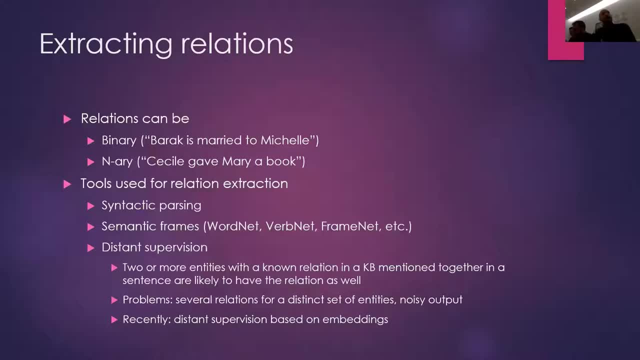 Now I can make some queries to extract New relations or next, like the new entities. Am I right or am I wrong? Yes, I think so. I don't know much about Wikidata, but they have to have something if they, of course. 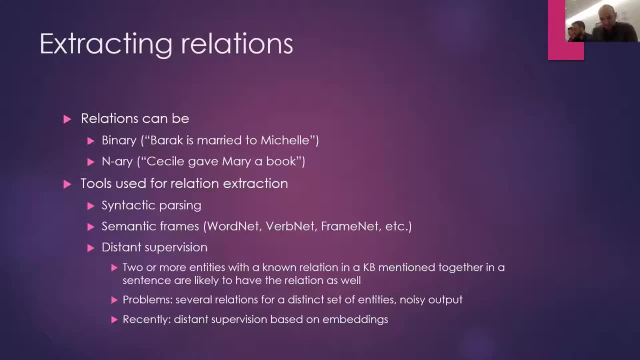 They are constructing a graph in the behind the scenes? Yeah, But for you guys- I think you would- You would probably want to either extract a sub graph of Wikidata That's only relevant for you, or like construct your own. I think that's the best right. 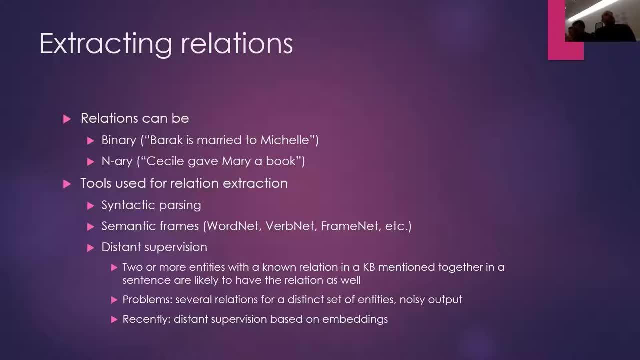 Yeah, because most of the vocabulary I'm using, Because of some I don't know. I don't want to go to the details, But most of the vocabularies I'm using up, like, let's say, today I had to, let's say, 30 percent. I found like one corpus and I had 30 percent. I didn't have the 30 percent of the Wikidata right. 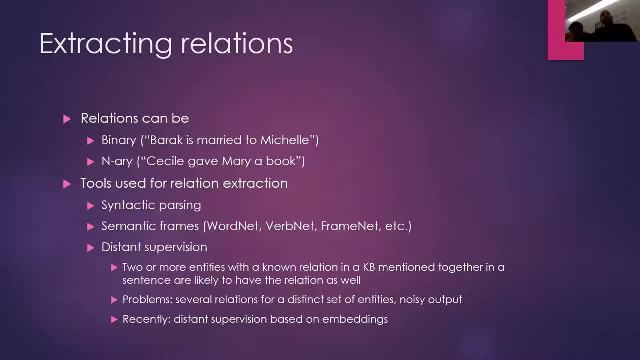 So I'm losing 30 percent work, work, embeddings, which I should create it myself. So if I'm gonna go it for the 30 percent of it like vocabulary, So better to do the whole like at least I have the whole knowledge myself, right? 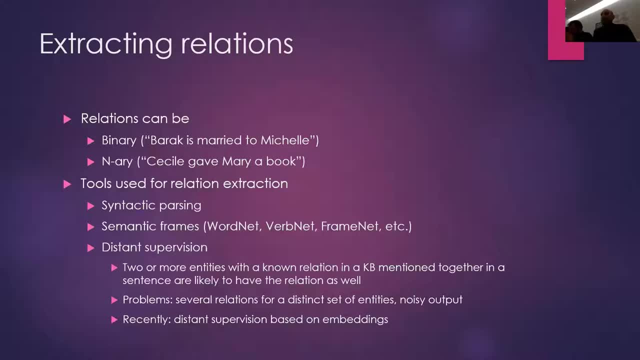 Then I have also extra knowledge that I don't need them. Let's say I don't, I'm not interested in the chemistry, We are interested in finance, Right, of course, the one, one approach might be Creating knowledge graph: first, create a, create a platform, then to the 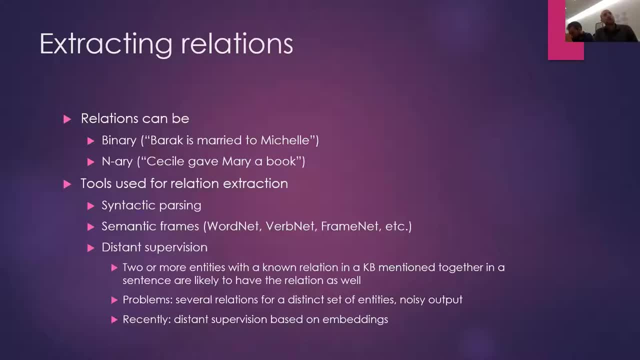 platform, going to go to create a Knowledge graph through the platform, similar something like what's Wikipedia already? Yeah, and I think there are ways to help you, like you don't have to do it manually. obviously, all of it, right. you could Extract all kinds of relationships from your corpus and then you could try to cluster them and see, you know, 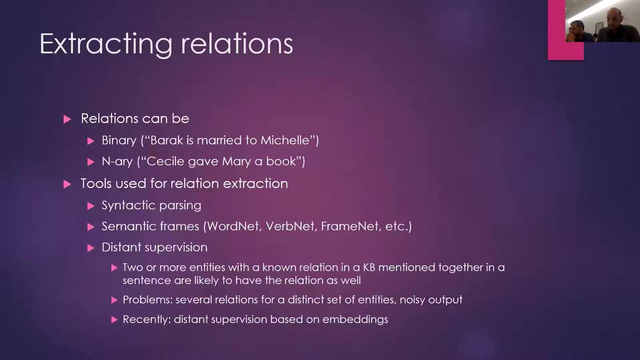 So use some kind of unsupervised methods first to help you Construct the knowledge graph. so Does that make sense? Yeah, that's yes, Thank you. That's what I was thinking Like. maybe I can do some sooty labeling a student relationship, but at the end of the day, I think the human should. 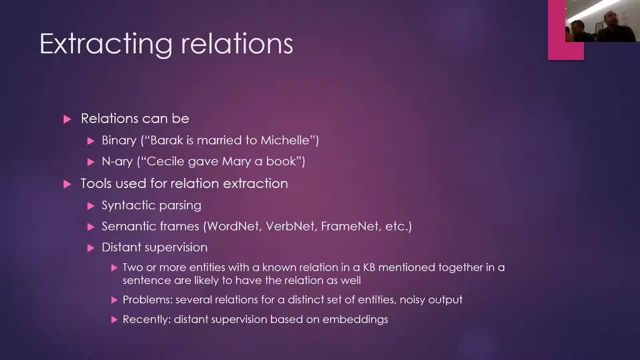 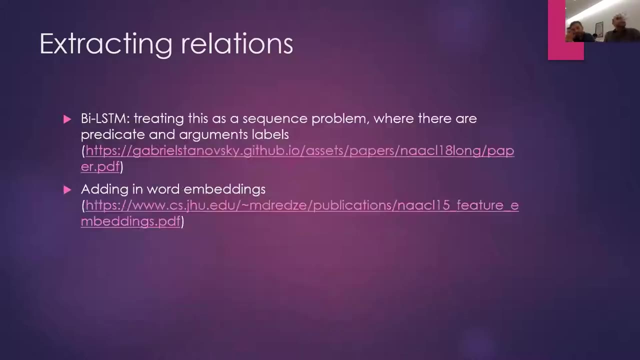 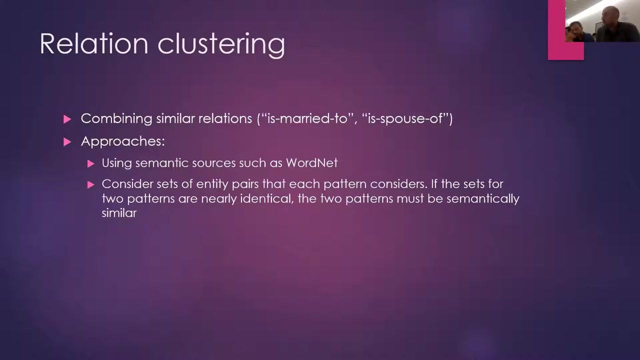 Check their relationships right, Yes, Yes. So first, like, do unsupervised and and suggest to the human and say, see, this is what we discovered. What do you think it's good And what is not good? basically, yeah, okay, thank you, sure, okay. so then you can do also relation clustering, because you know you have. 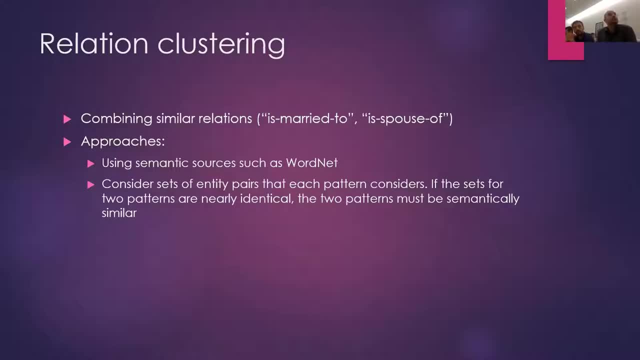 similar relations, such as is married to or is spouse of, are very similar. so um one approach is you can use semantic sources such as word net and frame net. um. the problem with those is that i think they're only english um, and they're very um. they don't include all relations um. 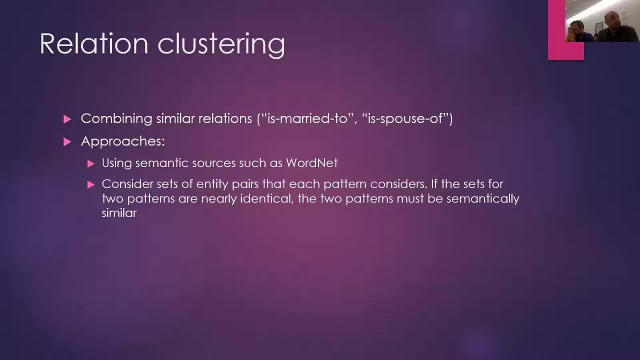 uh. or you could also consider sets of entity, pairs, uh, that each pattern considers um. so you could look if entities for the relations relation, the two relations, are the sets of entities. if they are nearly identical, then the two patterns must be semantically similar. so if you look at, is married to, usually it's uh, uh, a person's, two people's names, right? so, uh, if you. 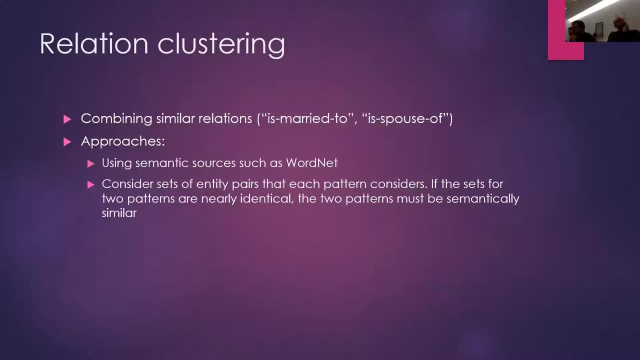 have two people uh is married to, it could be clustered with is spouse of, because they're also two names. obviously it comes with certain problems because two people is is married to and is spouse of is not. uh are not all the only two relations that uh use two people as entities. so 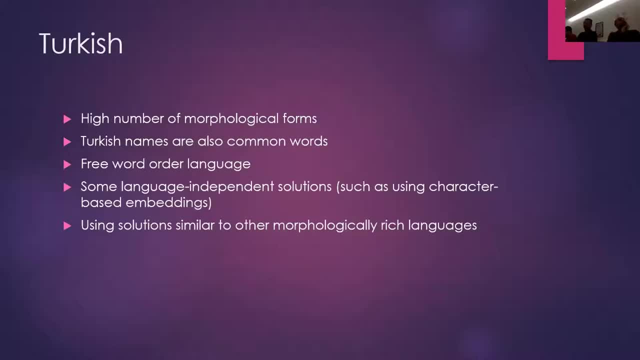 um, okay, so so i just you know just as uh, a few things about turkish. specific problems is that turkish has high number of morphological forms and, uh, what i didn't know is that turkish names are also common usually. uh, it's very interesting. so i guess that's a problem sometimes for named entity. 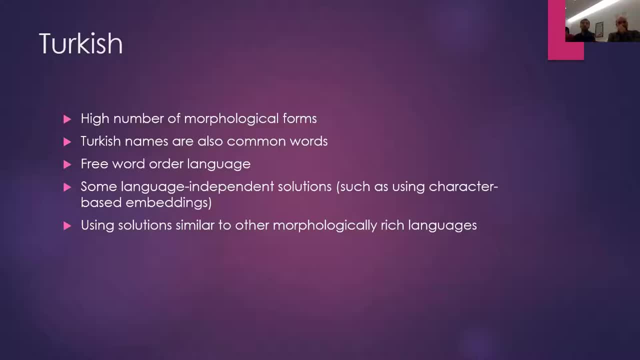 recognition and it's a free word or language like russian, so that's a similarity and so there are some like there's multiple confusion and then people choose words where you have a clear point, can some language-independent solutions, such as character-based embeddings, and also you. 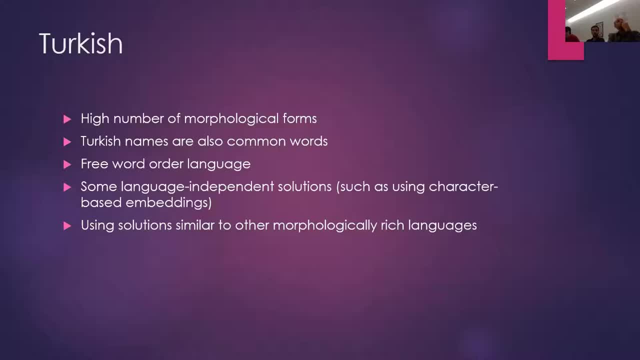 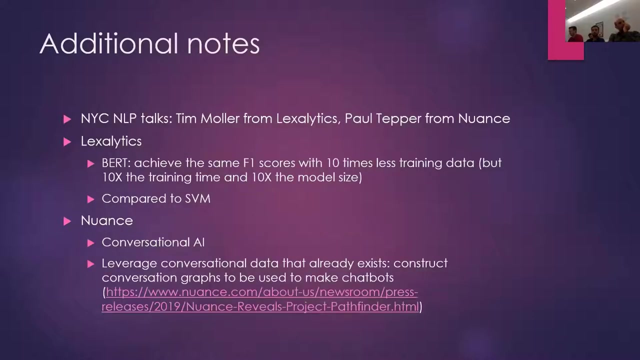 could use solutions that are similar to other morphologically rich languages such as Russian, And in the references section I have several papers that are specific to Turkish. You will see there's a section. Okay, so, as I said, yesterday I was at a NYC NLP talk and there's 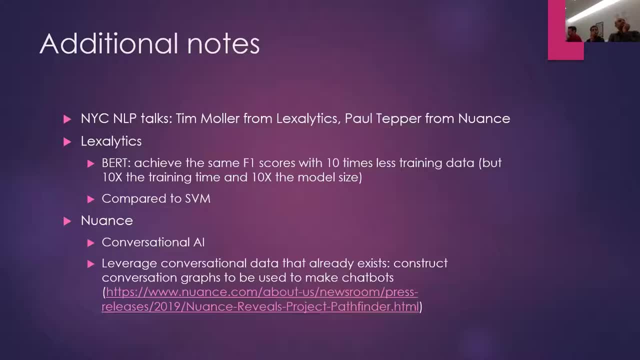 some things that might be relevant to you guys. I'm not sure, but maybe So. this company, Lexalytics. they did a comparison. They compared the task of classifying- I think classifying- movie sentiment into positive, negative or neutral and they compared the training time. 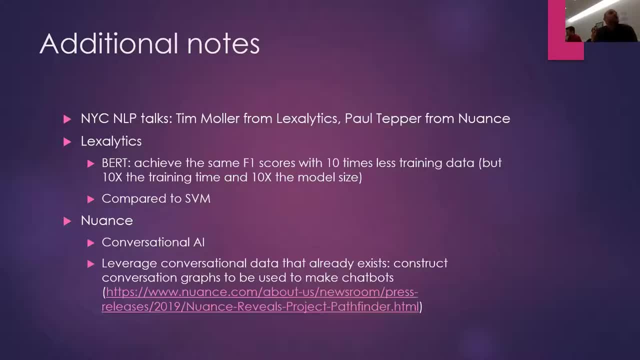 and the model size and the F1 scores between the two. So I mean SVM and I think maybe SVM with BERT. So BERT is the latest Google language model and what they achieved were the same F1 scores with 10 times less training data. 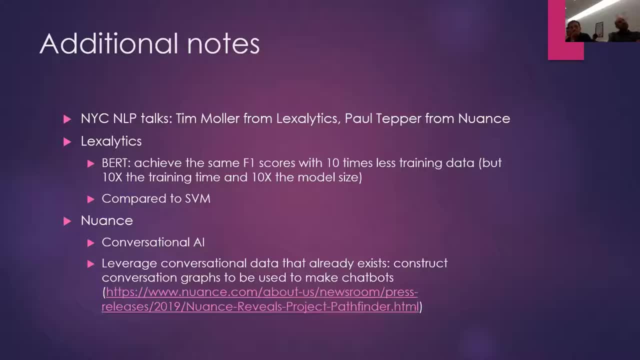 compared to just pure SVM. But also it's 10 times more. the training time was 10 times more and the model size was 10 times more, But I think it's an important note that you could use 10 times less training data for. 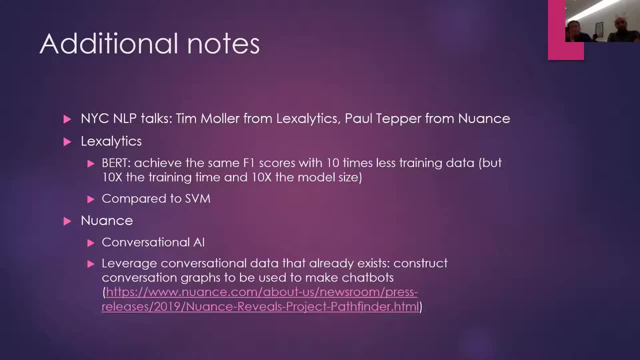 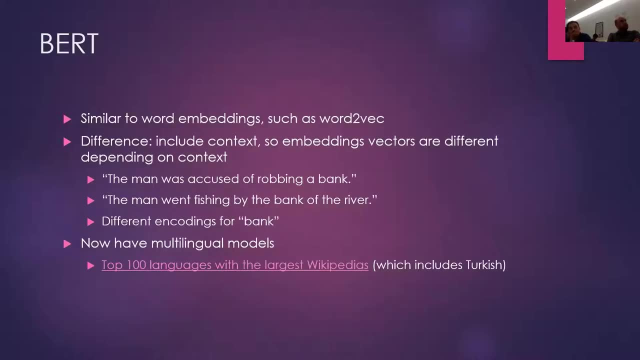 the same type of task and achieve the same type of result, And okay. so actually I have some stuff about BERT here. So it's similar to word embedding, such as Word2vec, but the difference is that it includes context. So the man was. 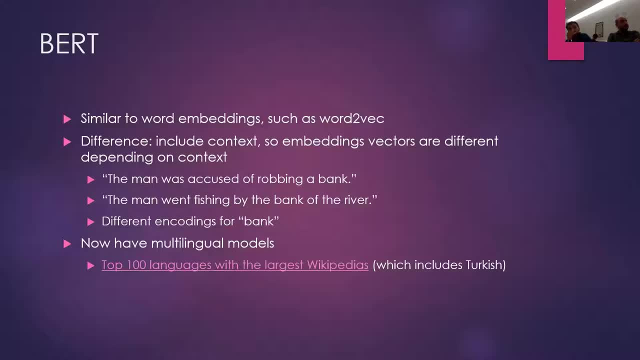 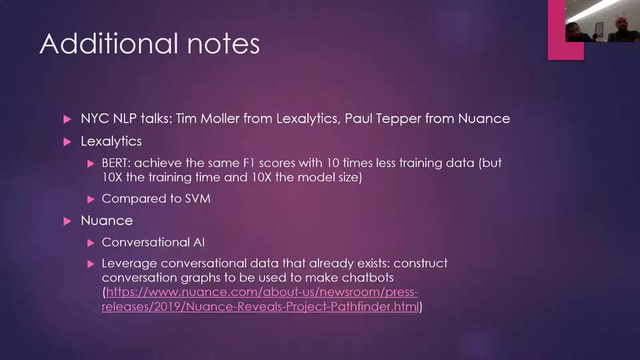 accused of robbing a bank and the man went fishing- fishing by the bank of the river. the word bank in the two sentences will have two different encodings and they actually have multilingual models that include top 100 languages with the largest Wikipedia's, which is, which includes Turkish. and another talk was 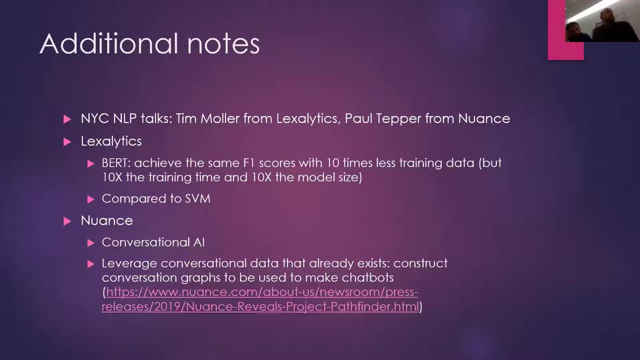 for conversational AI, so it's for designing chat, chatbot, dialogue flows. so what they did was they leveraged conversational data that already exists, so they had scripts of people calling into call centers to help with something like I think it was with also actually banking products. it was, for instance, 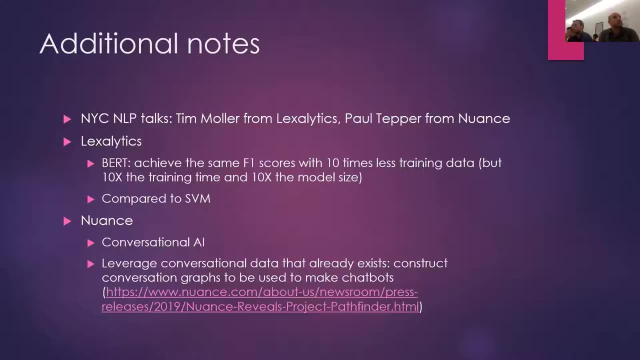 people calling and saying I want my credit line increased or I lost my credit card and they had. they graphed that data, basically so, with each turn being a node, and they clustered similar, similar utterances together so that they could show like: here are the possible ways. 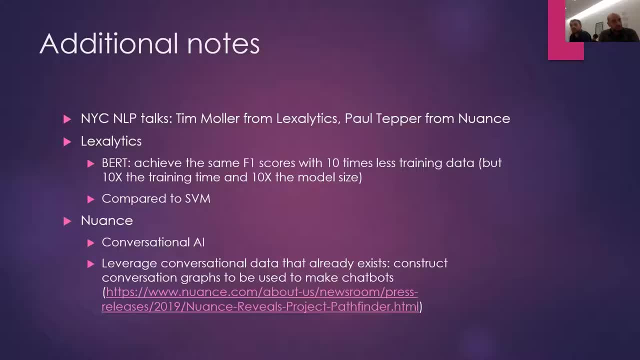 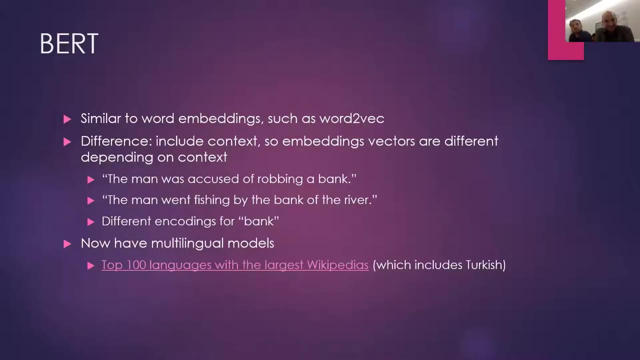 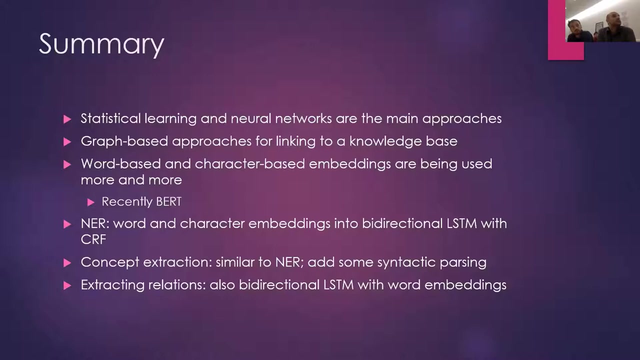 that this dialogue could go and it's a huge graph and you can filter it on different, different parameters. so you can read about it in the press release if you'd like. it was pretty cool, so ok, so we talked about actually the main trends basically are statistical learning and 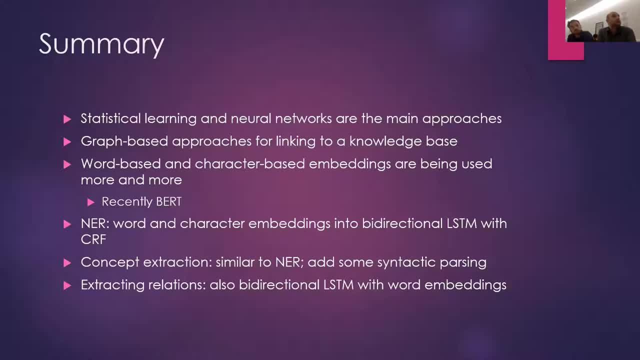 neural networks. there are main approaches and for knowledge basis, graph based approaches are the most popular ones, and word based and character-based embeddings are being used more and more, and BERT and my lab is not a lab, so we have to have all the data to supervise it. 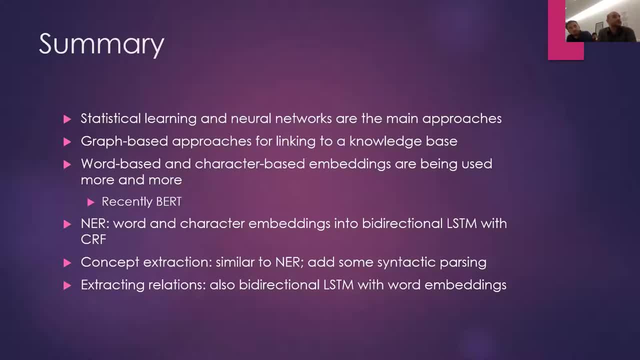 recently, which takes into account context, basically, And NER, basically the state of the art, is word and character embeddings that are fed into a bidirectional long short-term memory network and then into a CRF. So concept extraction is similar to NER. add some syntactic. 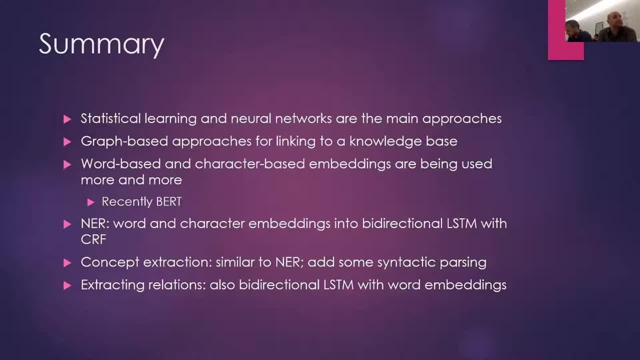 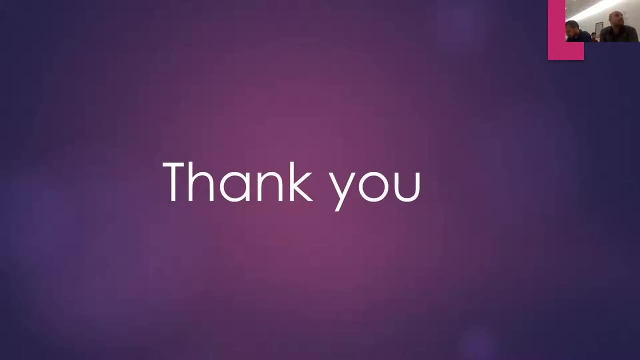 parsing to identify noun phrases and extracting relations. also, a bidirectional, like the state of the art, is the bidirectional long-term memory network with word embeddings. So basically that's it. Thanks a lot, Let's check if somebody has a question. Okay, thank you. Any other? 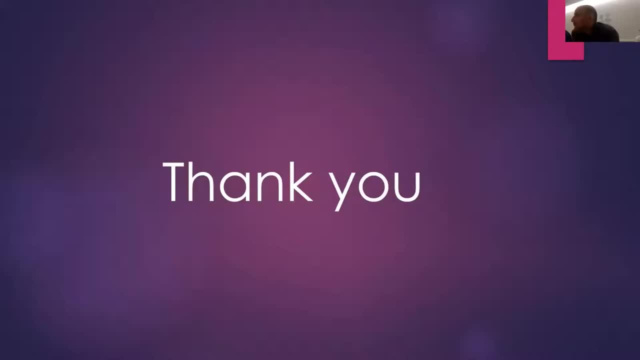 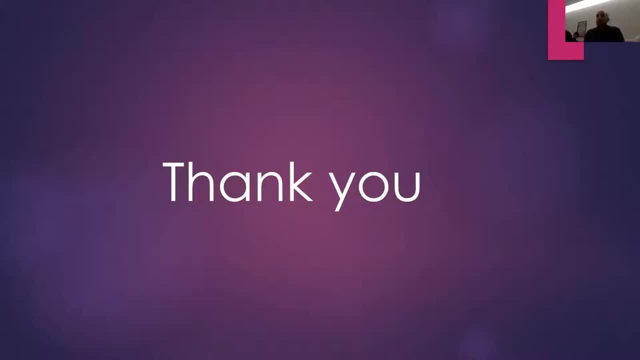 on. I might bother you but later, but thanks a lot for giving us this opportunity And it was great. literature review and theory about and I learned a lot about the theories- new theories and what, how to use them, how to use them and how to use them and how.